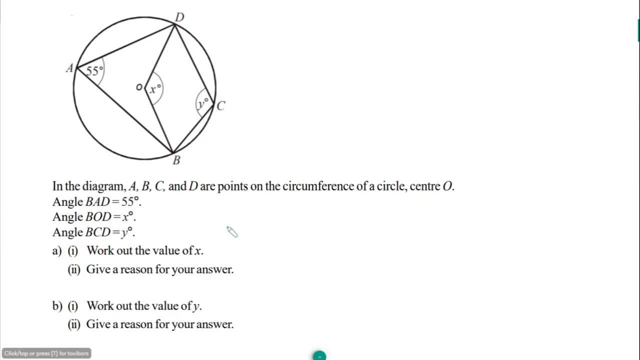 Hello everyone and welcome to the second part video on circuit theorems. In this video I'll be walking through numerous kinds of questions you can find on circuit theorems. Some gonna be simple, some gonna be difficult, some gonna be mid-range. Now it doesn't matter what kind. 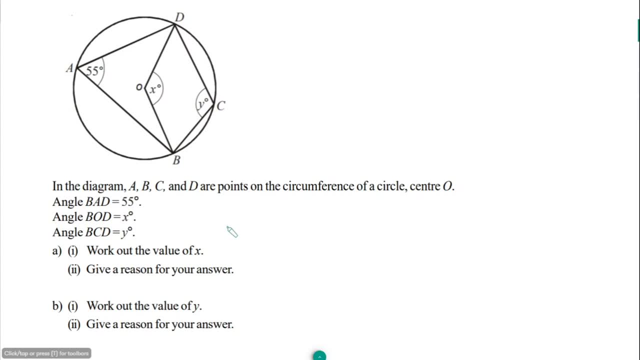 of question you find here. at the end of this session you will have a better understanding on circuit theorems. So without wasting any of your time, let's dive in straight into the first question Now. here we have a diagram- A, B, C and D on the point of a circle or 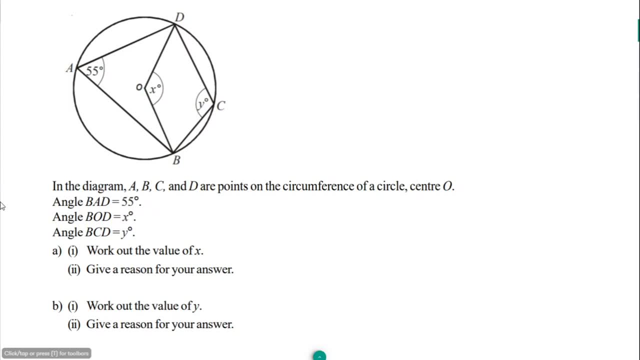 its center O. Okay, center O here. and angle BAD is 55 degree and BOD is X degree. Okay, and then angle BCD is Y degree. Now, in the first part question we ask to find the value of X. Now, this is angle X here. Okay, to find the angle of X. now we can consider this. 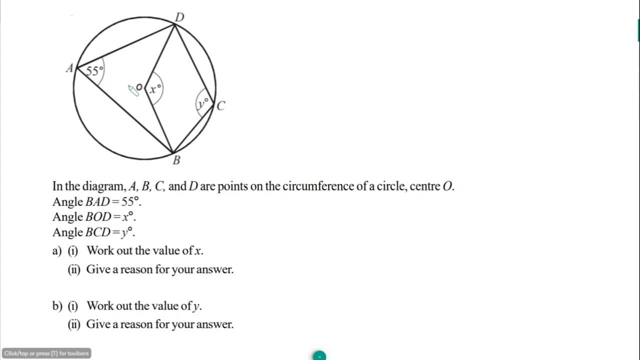 angle of the circumference here. Definitely it has to be twice the angle here. So if here is 55 degree at the circumference at the center, it has to be twice of it, And then it's going to be 55 times 2.. So to work out the value of X, I can say X is going to be. 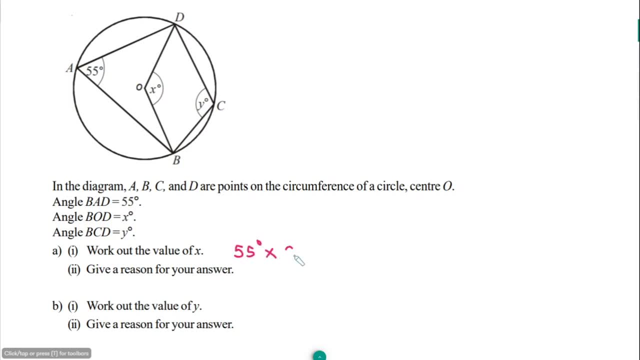 55 degree times 2 and this is going to give me 110 degree. So angle X is 110 degree. Now the reason here we ask to find the reason. So give me a reason for your answer. What is angle Y? Well, angle center, okay. Angle center of a circle: okay, Angle center is. 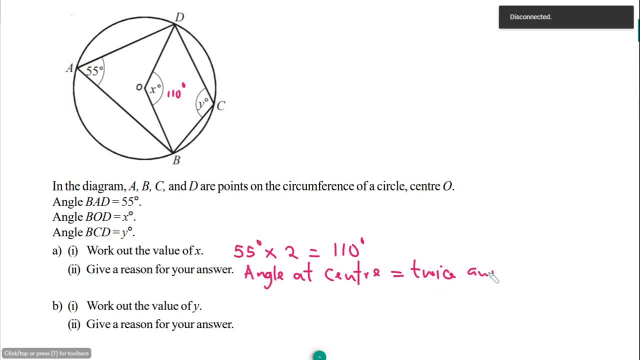 equal to twice angle at circumference. Okay, That's make it very easy Conference okay. Now for question B. it says: work out the angle Y- Yeah, this angle Y, Okay. And to find angle Y you can consider two ways you could do that. 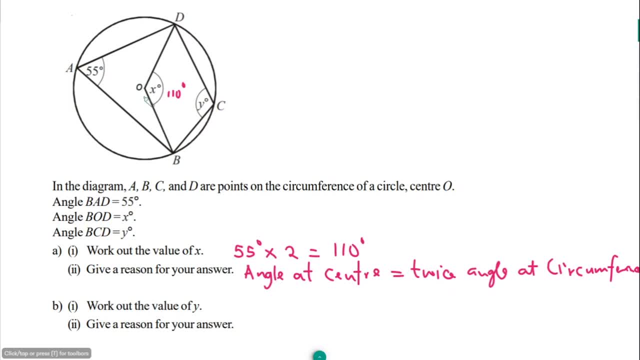 1. to try to find the reflex angle here and then divide by two to get angle y, or you may consider that this is a cyclic quadrilateral. 55 and y should add up to 180 degree. any of these two steps you use, you arrive at the same answer. but i'd like to use the opposite angle of exactly. 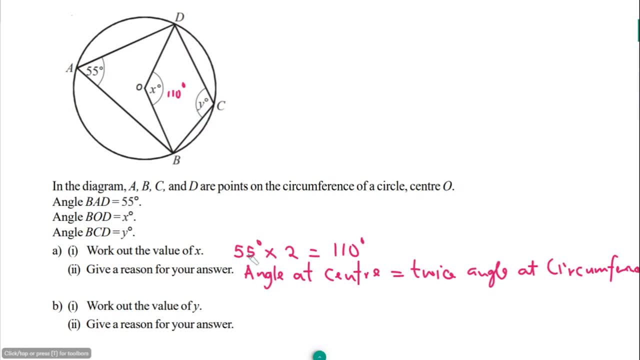 quadrilateral. okay, so it means 55 plus y should give me 180. so to get y, what i need to do is to say 180. okay, i'll subtract 55 degree and if i do the subtraction i'm gonna have 125 degree. okay, that's very easy. so y definitely gonna be 125 degree. okay. now question i. i says, give a reason. 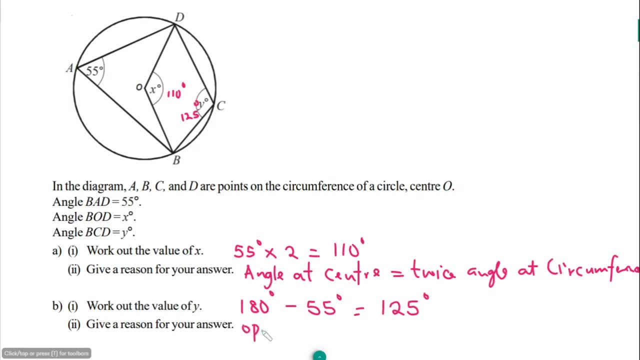 for your answer. well, the reason is the opposite. um, opposite angle, okay, opposite angle of a cyclic, opposite angle of a cyclic. opposite angle of a cyclic, collateral cyclic- how about gonna spin right, good, cyclic quadrilateral, okay, add up to add up to 180 degree. so that's very simple, okay. so now we're going to move to the next question. 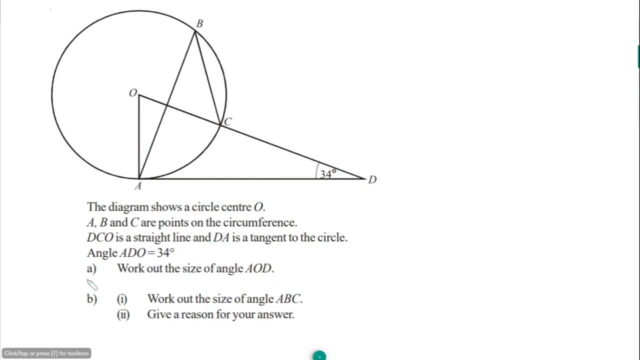 yeah, we've got a diagram here and that shows the center, o and abc. a point on the side confrontations. now, DCO is a straight line. okay, so this is DCO on a straight line and DA is a tangent. so D is a tangent to the second and angle ADO is 34, so that's 34. 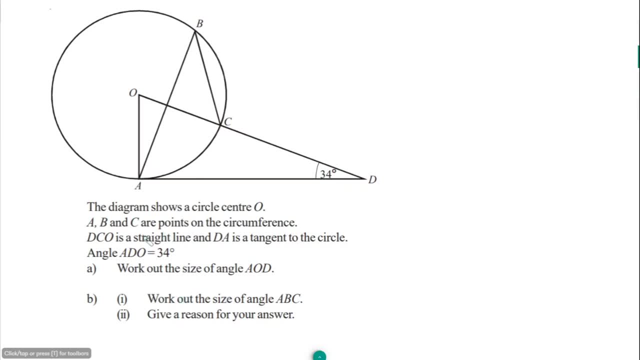 degree. and now we need to work out the angle, AOD, and so this is AOD. okay, so this is the angle we're really looking out for. okay, I'm gonna shade it to make you see it very clearly. okay, now to find that angle, we need to consider some. 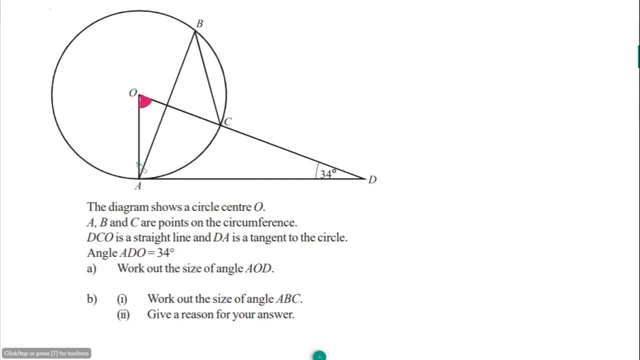 theorems. now, this is a radius and this is a tangent. remember we said for a tangent meeting, a radius it means that always be the 90 degree. that means this angle here is 90 degree. so if you consider this triangle here, that's angle AOD, 90 degrees plus 34 plus this angle should give you 180, because sum of angles. 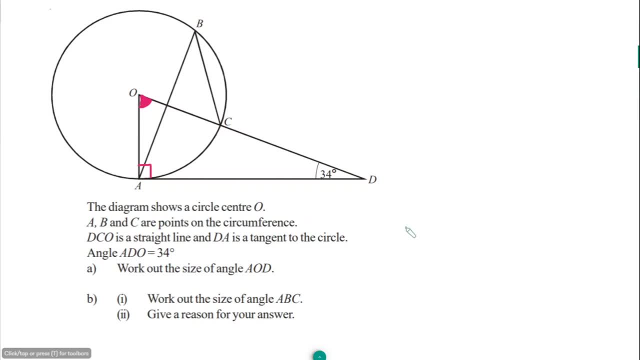 triangle is 180. so what I'm gonna do here right now is say: I'm gonna add 34 and 90. okay, 34 and 90, that's gonna give me 124 degrees. I'm gonna subtract that from 180 degrees and that's gonna be 124. I'm gonna subtract. 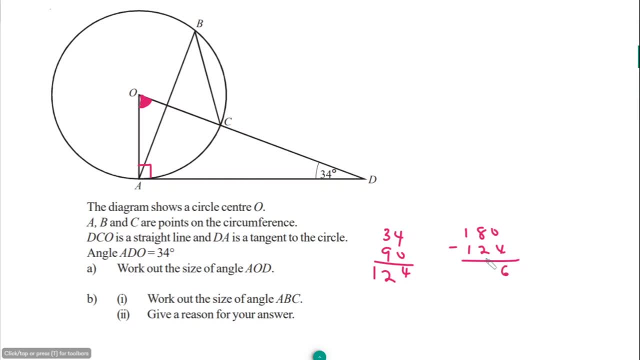 okay, and that's gonna be 8 minus 2, 6 over 5, okay, 56. so that means angle here is 56 degree, okay, so this angle here is 56 degree, okay. now, of course, here, and this is the great update here, okay, now question basis: what are the? 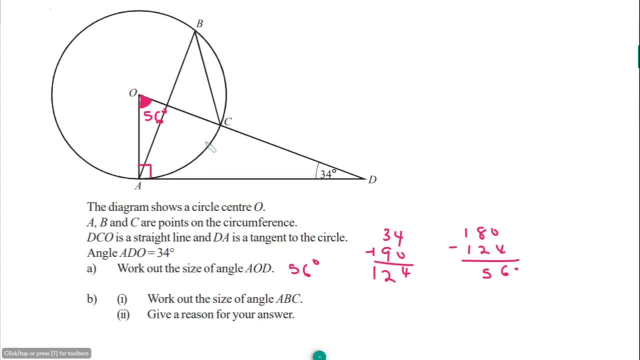 size of angle ABC. now, angle ABC really refers to hear. okay. so this is the angle we are kind of looking out for now. to know what I need to look for, always check the middle letter in the giving alphabet. that gives idea what you're going to be looking out for. okay, so if he is 56 at his side, 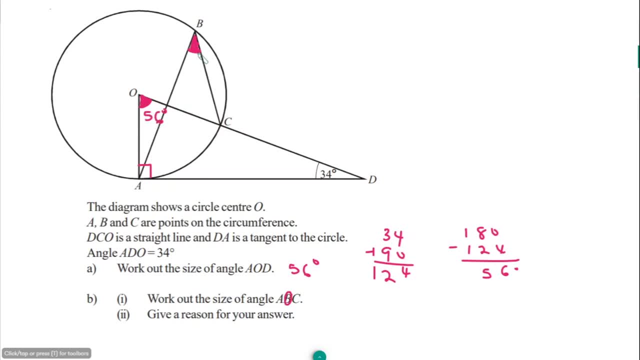 Okay. so if here is 56 at his side, center at a circle is gonna be half of it, okay. so angle: angle ABC is gonna be 56 divided by 2 and that's gonna be a 28 degree. okay, so this angle is definitely gonna be 28 degrees. so okay, and for question II says: give a reason for your. 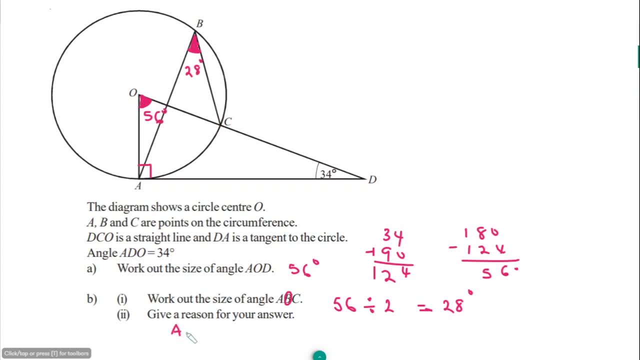 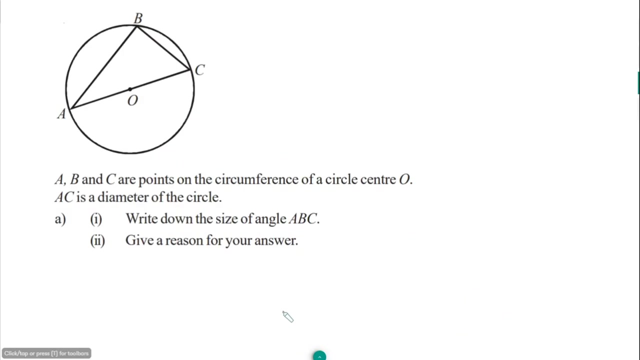 answer. well, the reason so is quite simple: angle center: okay, angle at center is twice the angle. it tries to anger at the second phrase. okay, okay, just make it very quick. all right, so that was very easy. so we know the angles for ABC and, of course, reason: okay, so let's move on to the next question. now we have a set. 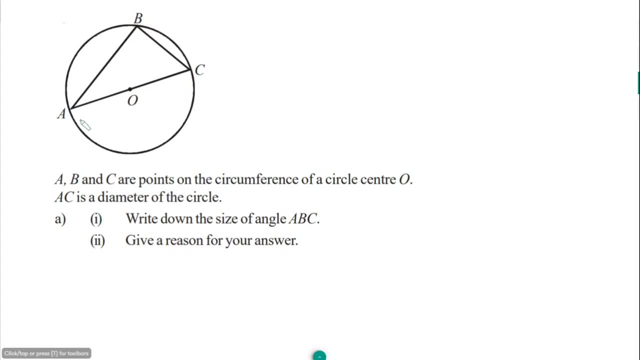 we haven't died up here. and ABC at points under circumference of the circle with center o and ac is diameter. okay, very, very instructional ac diameter. so question a is right on the size of angle abc. so i'm looking for the angle on b. so there's definitely this angle here, all right. 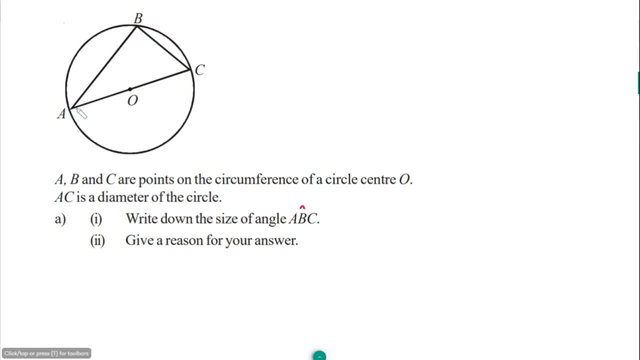 now, since i know, having told that this is a diameter ac and this is um angle, this angle on the semicircle, definitely this angle has to be 90 degree, okay, so it's a right angle, really. so angle abc, the size of it's gonna be 90 degree okay. 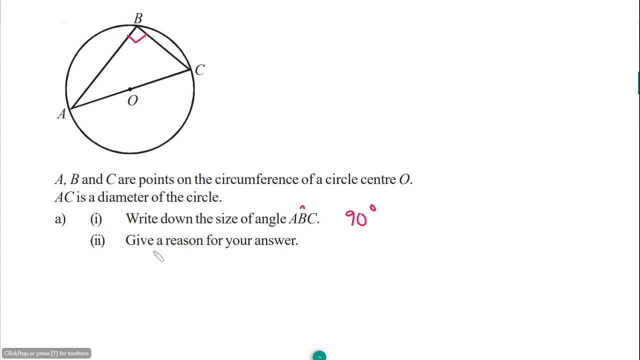 and questions the question that follows after. it says what's the reason for your answer. well, it's very obvious. angle: the semicircle is 90 degrees, so you can say angle at the at the semicircle. okay, semicircle a is right angle. okay, that's. 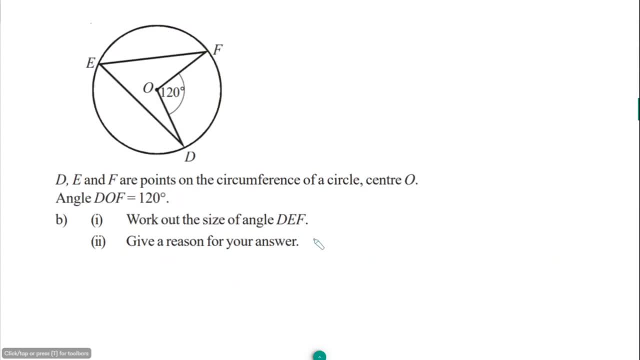 very easy, okay, so let's move on to next question now. angle def, our points on the second frame of the circle with center o. okay, we have it there, and angle dof is 120 degrees. now we need to walk out the size of angle d, e, F. remember, your focus is on. 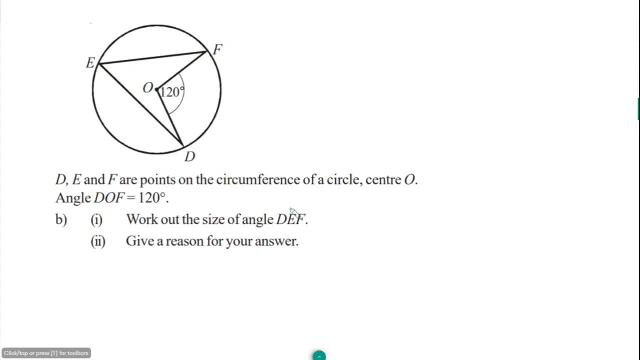 the letter in middle between df and s, angle e. so I'm gonna look- this is where I'm looking at for- and good def here, okay. I'm going to look for angle where the okay, good now, okay now. so what i'm going to do here is um, if here is 120 degrees, definitely. 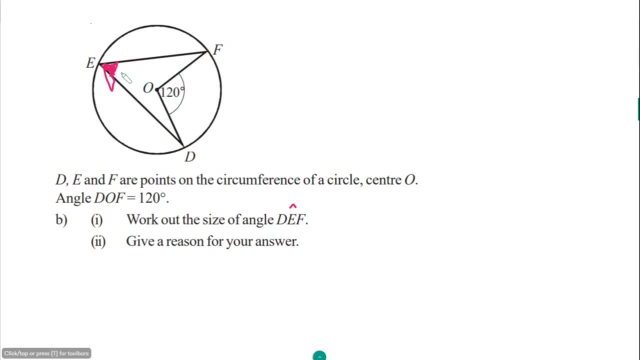 this angle is going to be half of it, because angle center is twice the angle at a circle. so this angle is going to be 120 degree, uh divided by two, and that's going to give you 60 degree, okay. and the second part, give a reason for your answer. well, angle center, angle center is uh. 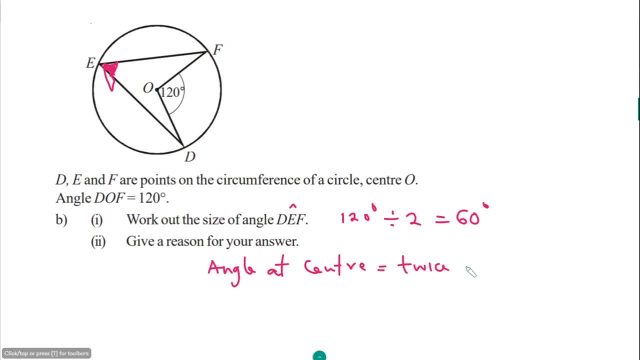 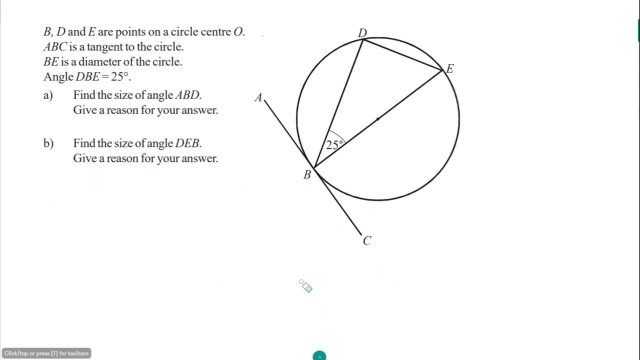 twice the angle. twice the angle at the circle of friends. does the angle at the cycle of friends? okay, so that's it. okay, let me just wipe this out to make this a little need to. okay, all right, and now we move on to the next question. now this looks a little bit. 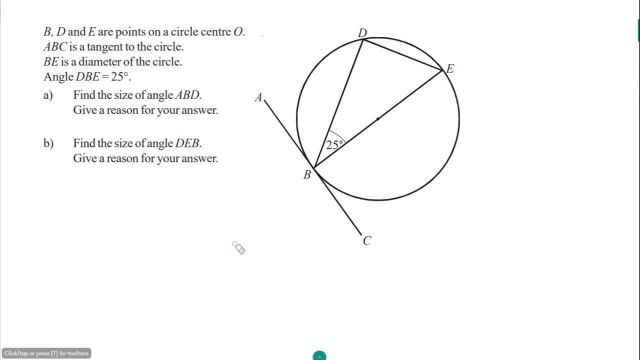 complex, but it's very simple. but let's look at this question first of all. let's look at it first of all. you, I'm going to be somewhere here, center, oh, okay, and a, b, c is a tangent. okay, this is a tangent. and b is a diameter. b is a diameter and angle d, b e 25 degree. good, now the question says: 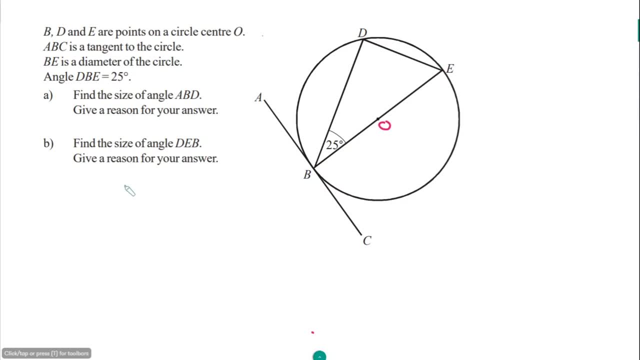 find the angle size of angle a, b d. a b d is definitely going to be somewhere here, because a, b d, okay, now to find this angle, okay. one thing we can consider, uh, first of all, is: um, you, you could think, you, you could think this as a straight line, okay, and then you have your tangent. now, remember, 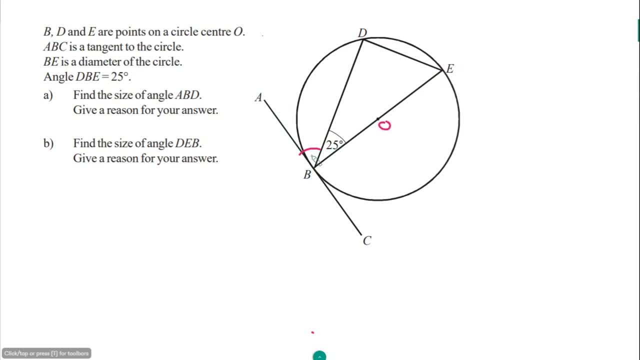 these two angles, this angle tangent and straight line here- should add up to 90 degrees, okay. so this whole part here, okay is 90 degree and I know here's 25 and I need to find this angle. all I need to do is to subtract 25 from 90, okay, so I'm going to do something like this here. so I'm going to do 90 degree. 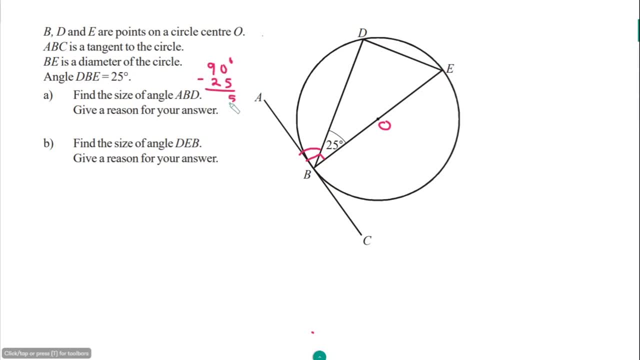 minus 25 degree and that's going to give me 65 degree. okay, so this angle here, angle a, b, d- I'm going to show that so you can see what I'm really referring to especially. okay, that's this one is, uh, 65 degree and reason: okay, the reason is very simple, you know: radius. 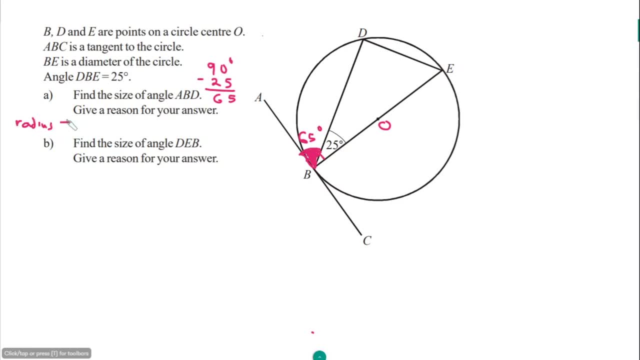 on radius and tangent register. tangent is um 90 degree, okay. and then question b says: find the size of angle d e b, d e b. all right, um d e b is going to be somewhere here. this is the angle I'm looking at for. okay, all right, now this angle here is: is is as alternate segment to this angle here. okay. 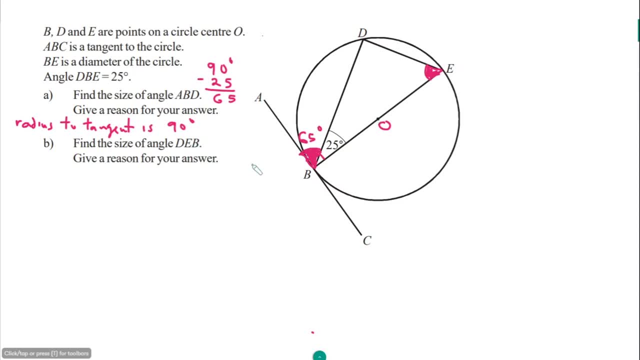 okay, so the angle d e b is definitely going to be 65 degree also 65 degree also here. the reason I'm going to turn a segment equal, okay, autonomous alternates segment. the segment angles are equal. okay, that's very easy. so here's gonna be 65, all right, so that's done. so we go to the 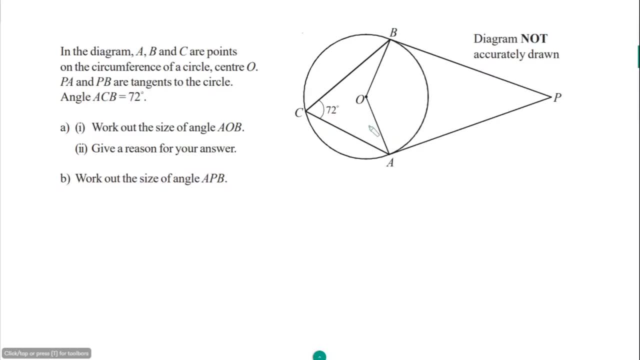 next question: all right, and this diagram, ABC appoints on the second first of a second with Center O and PA and PB are tangents to the cycle, okay, and angle ACB is 72 degree and then we need to work out the size of angle a OB. I will be. 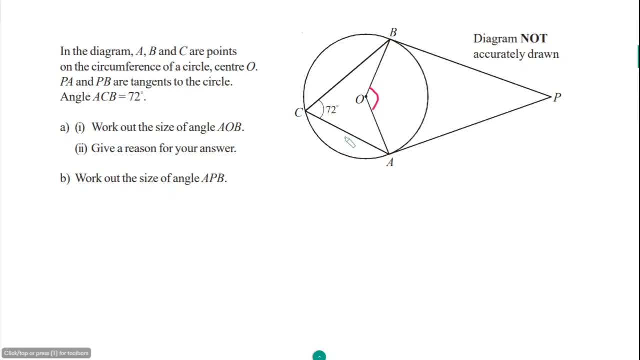 definitely gonna be here. well, that's very easy to find because if he's on the two angles centers twice the angle made as a circumference. okay, so here's gonna be 72 times 2. 72 times 2 that's gonna give me a hundred and forty four degrees. so this time here is gonna. 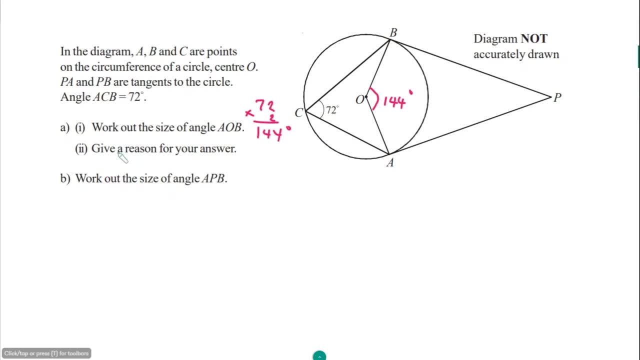 be a hundred and forty four degree. the reason is angle. Center and go Center is twice anggio, twice angle as circumference, twice angle at 게. good, now for question pieces. what are the size of angle? a PB, EPV is actually the angle here. okay, so we got for these angle here, but I'm trying to give it a shade. okay, a good one here we. 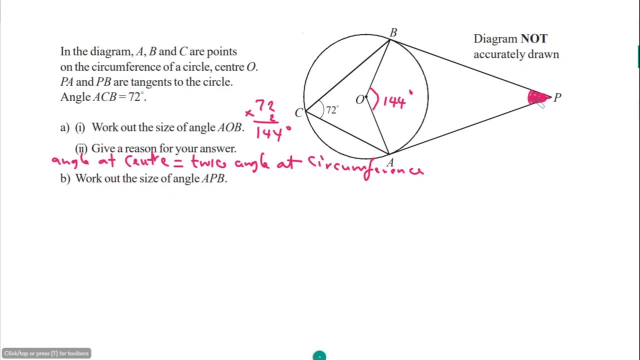 Now one thing to find this angle: APB, we already know that we've been told that this line tangent here and this tangent meet at P. That suggests that remember the term we said that when you have two tangent drawn out to meet at a point, the tangent should. 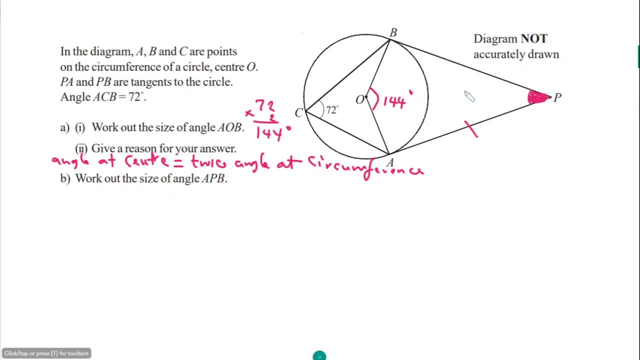 be equal. Definitely. that means this angle, this length here, the tangent here is equal to the length of this tangent here. That's very easy. Another thing we need to consider: we have a radius that comes from here down here and meets a tangent that's going to be 90 degree. 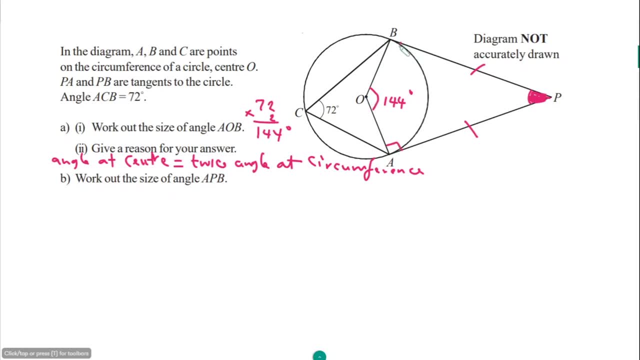 The same one on the radius meets another tangent here that's going to be 90 degree. So we got three angles and another angle here, APB. Now I know that I have what you call a quadrilateral here, And if I add up these four angles- this, this, this and this- I'm going to have 360 degrees. 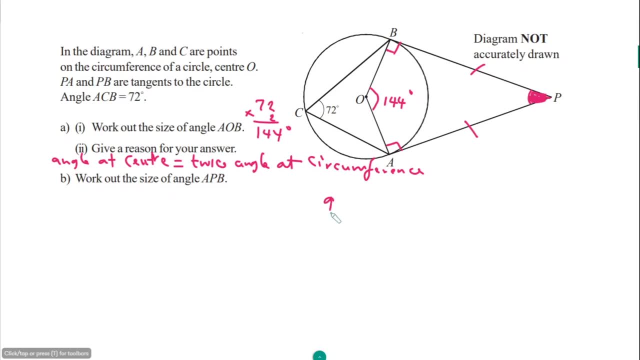 So I'm going to add these three angles first, and 90, add 90, that's going to give me 180, and add up 144, also 144, that's going to give me 324 degree. Okay, All right. 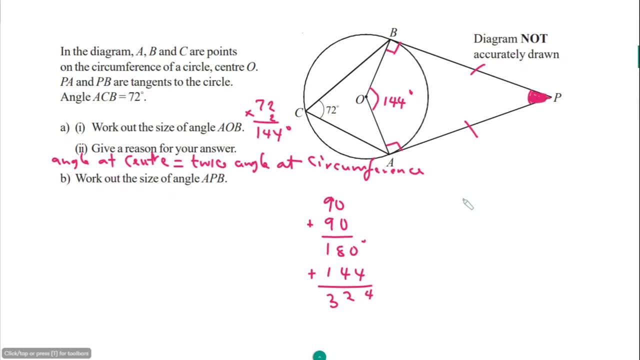 Then to find this: I'm going to subtract this sum from 360.. So I'm going to have 360.. So I'm going to subtract this sum from 360 degree minus 324,. okay, Now, if you do the subtraction, the subtraction, and you're going to have six here for 36.. 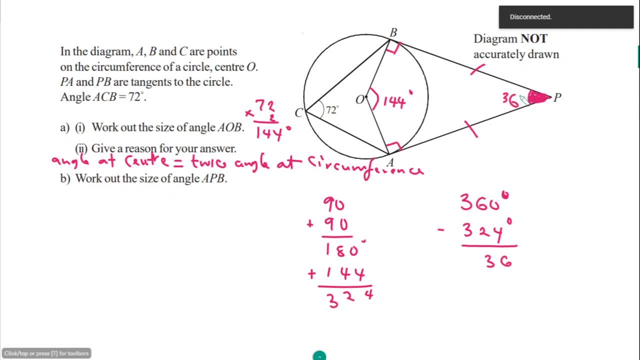 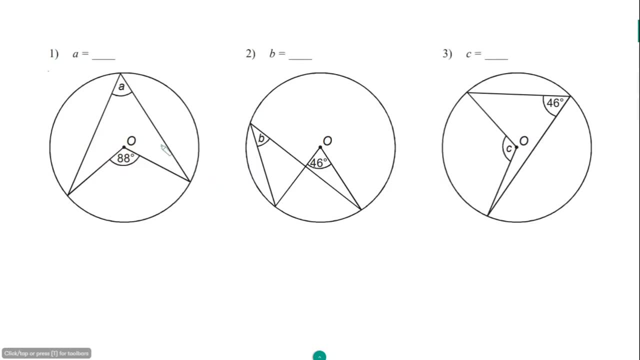 So this angle is going to be 36 degree, So that makes it a lot easier. right Here we need to find the angle mapped ABC. okay, For the different. Let's check the terms. Probably you have here Now, if you look at the first question here, um, we've got angle, middle and circumference. 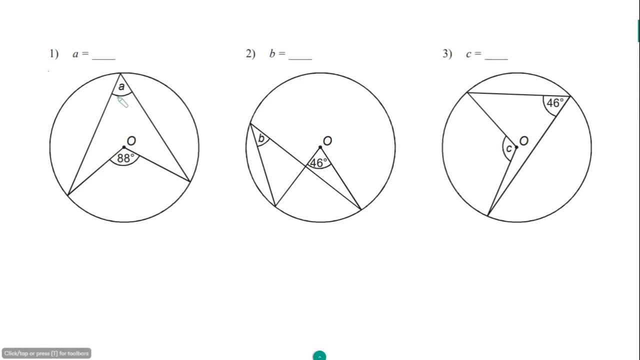 88 degrees and we need to find the angle made at the circumference. here a this is going to be if here's 88, because I'm going to center is twice the angle made at the circumference. So here's 88, angle A is going to be half of it. 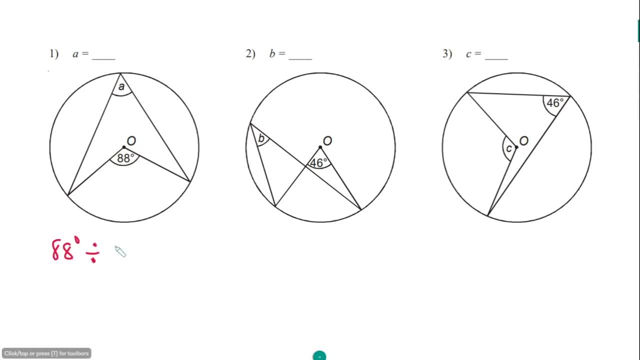 So we're going to have 88 degree divided by two and that's going to give you 44 degrees. So angle A is 44 degrees, Okay, And then we're going to question B, okay, number two, if here's 46 degree at center. 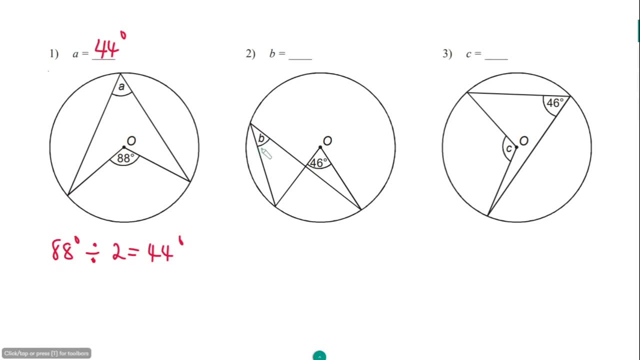 then we need to find the angle here, B at the circumference. Okay, I mean at the circumference, Okay. So well, let's do the same thing. We're going to have to do 46 divided by two, and that's going to give you 23 degree. 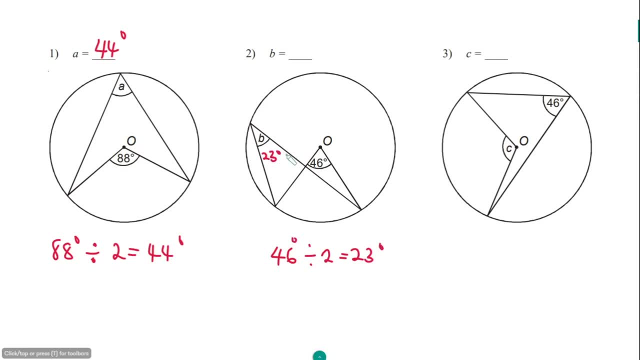 Okay, So here's going to be 23 degree, Okay, And so we come down here, up here, right, 23 degree, And then we'll come to question C. Okay, Number three, We need to work at the angles. 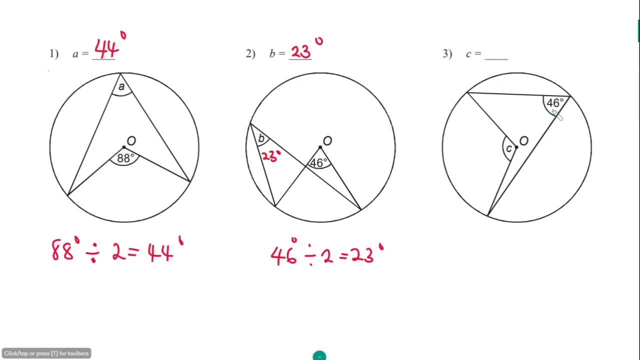 C at the center. If the circumference angle here is 46, at the circumference at the center, you're going to have twice of it. So it'll be 46 degree multiplied by two. That's going to give me 92 degree. 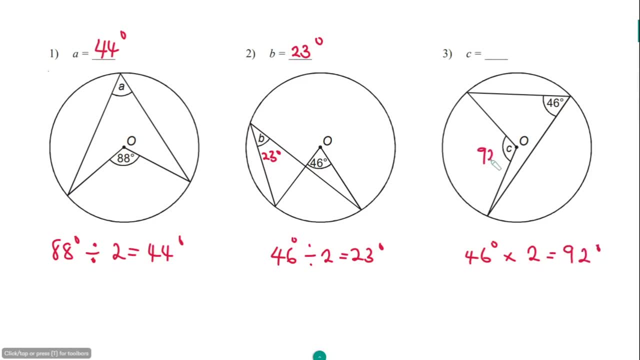 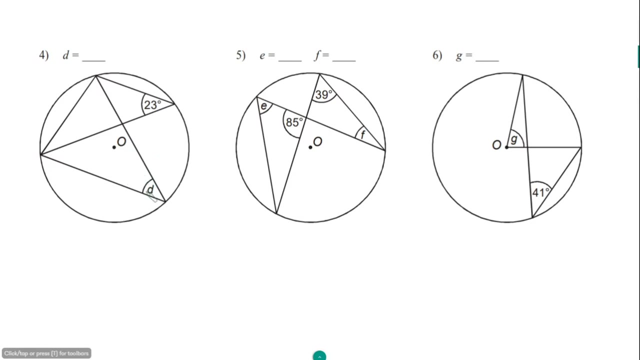 Okay, All right. So here's 92 degree. So C is going to be 92 degree. That was pretty easy, right? So let's move on to number four. Here we have a second Turing problem. Now we need to find the angle marked D. Well, if you really consider, 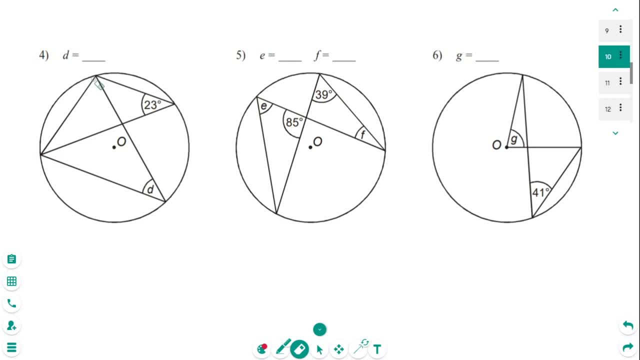 I want to do something here to help you see what I'm seeing If I try to move this line here. okay, you can immediately see that 23 is the same angle as D angle on the same segment. right, But I'm going to restore it back. 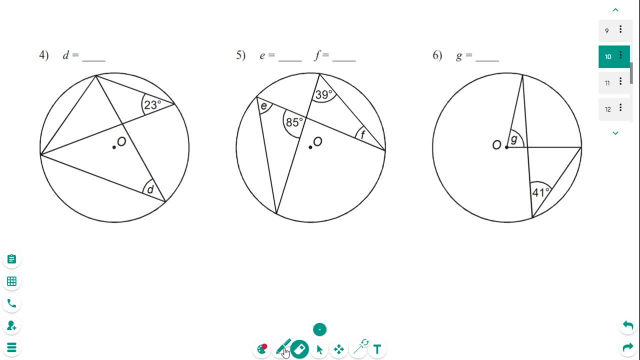 Okay, Just to help us see. Okay, So if it's 23,, D is going to be 23.. Okay, So D is 23.. The reason is because angle on the same segment are equal, Okay, And the same for number five. 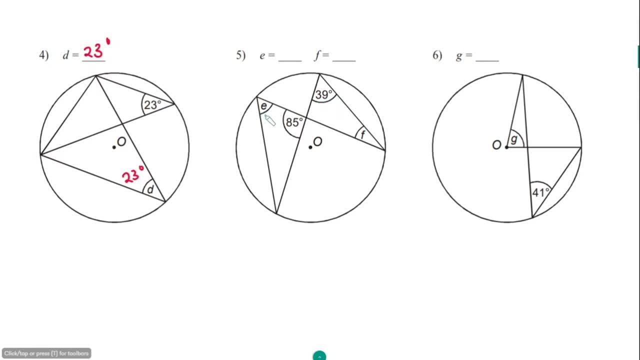 The same thing. If here is 39, letter E should be also 39. Angle on the same segment. So letter E is going to be 39 degree. So I'll come down up here. I'll write down 39 degree here. 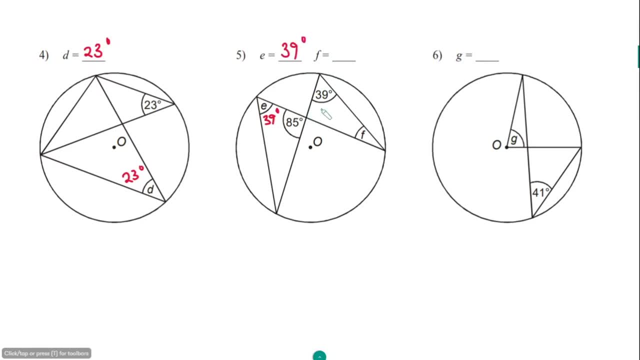 Okay, But I need to find angle F. Well, to find angle F, there are a couple of ways you can do that. Okay, F here is going to stay in the same angle here. Okay, Because there's going to be, you know, angle on the same segment. 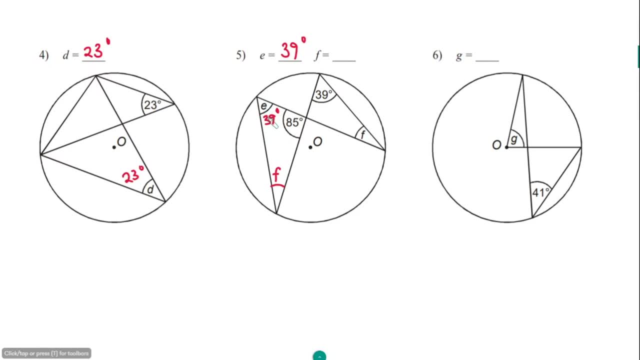 Okay, So I'm going to consider this triangle here. 39 is 85. And the result I want to subtract from 180.. So let me try it here: 39 plus 85 degree, And that's going to be 4 here. 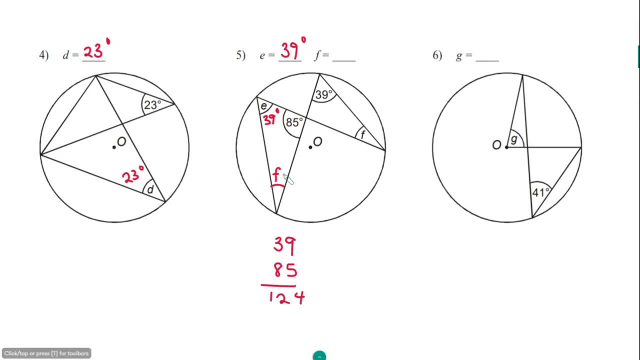 Carry 111.. 12. 124 degrees To find angle F. I'm going to subtract this from 180. Remember I did add here. So 180. Subtract 124. That's going to give me 56 degree. So that means angle F is 56 degree. 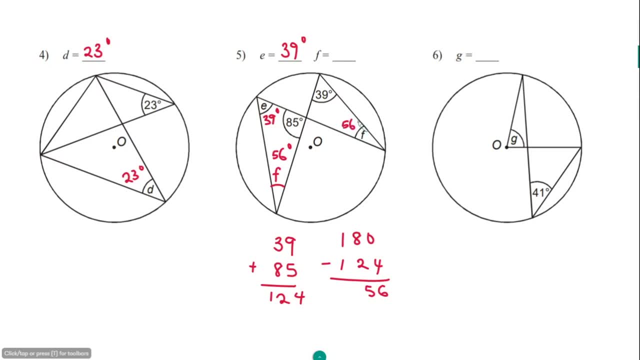 Mm-hmm And that's in here. So angle F is 56 degree. Pretty, very easy, Right, Mm-hmm. And then we come to number six. We got a drawing here. I have an angle here at the center. 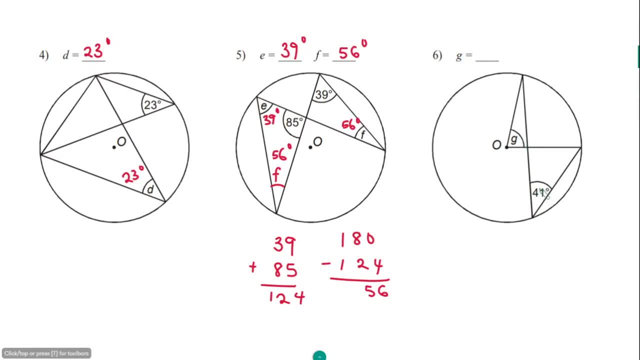 And an angle here at the second front. Well, still, the same. Angle at the center is always twice the angle at the second front. So if here is 41 at the second front, at the center, it's going to be twice. It's going to be 41 times 2.. 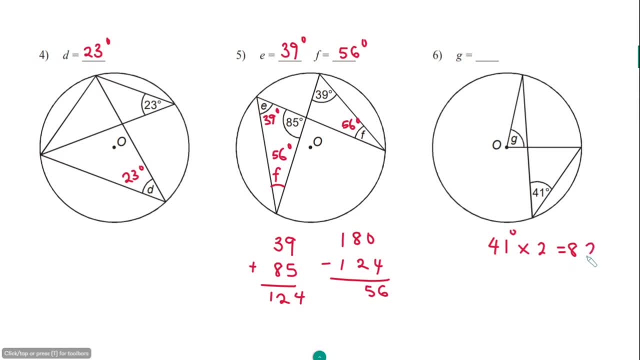 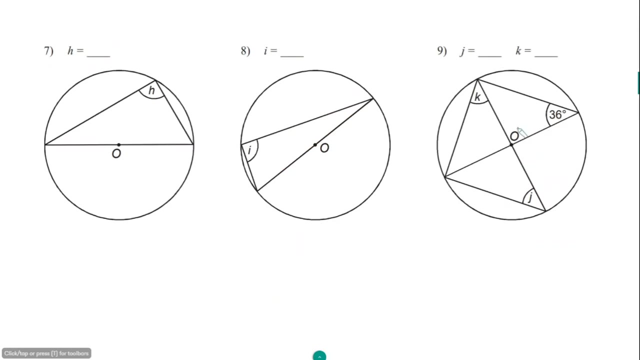 Okay, And that's going to give me 82 degree. So angle G, Angle G, is going to be 82 degree. Okay, Write it down. So I come up here: 82 degree. Very simple, Right? Okay, Let's move on. 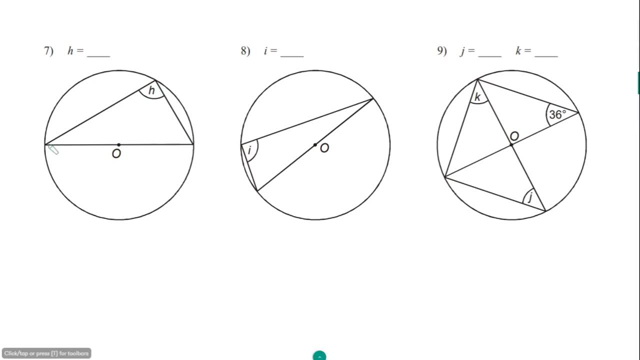 Let's see more. All right, We got an angle in the semicircle here And this line here is a diameter. Okay, We set to O. Now this obviously, angle in the semicircle is going to be 90 degrees. 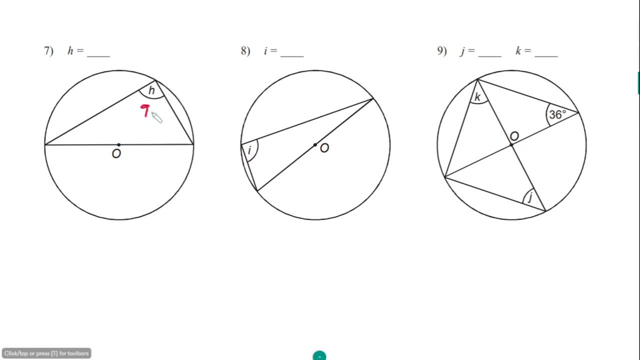 So angle H definitely has to be 90 degrees, There's no question about that. Okay, And the same for question eight: The same thing You can see. this line is a diameter passing through the center O, And this makes an angle at the semicircle. 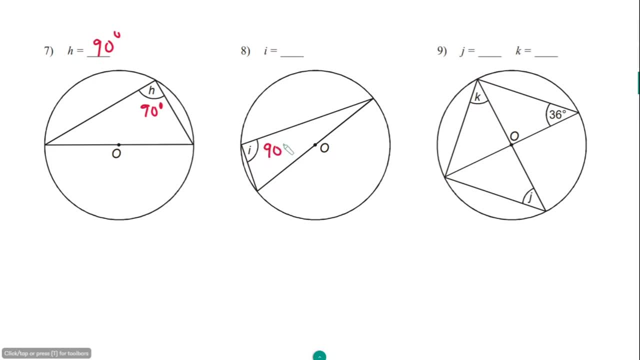 Okay, So the angle I definitely also going to be 90 degree. So angle here is going to be 90 degree. And then we come to question nine. Hmm, Now, if you look at this question, you can see she got two lines passing through the. 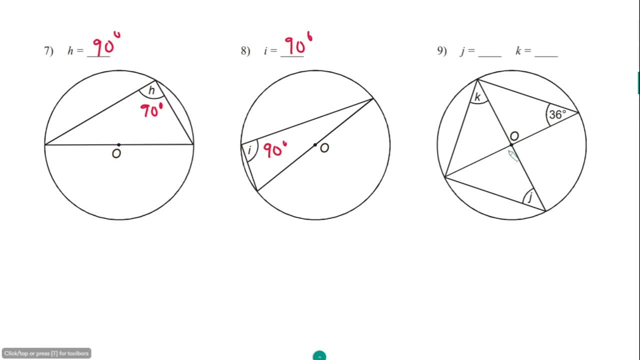 diameter, Okay, Through the diameter center O. Now I already know that angle G is going to be equal. Okay, So J is going to be equal to 36 degrees, because, well, that's going to be angle in the same segment. 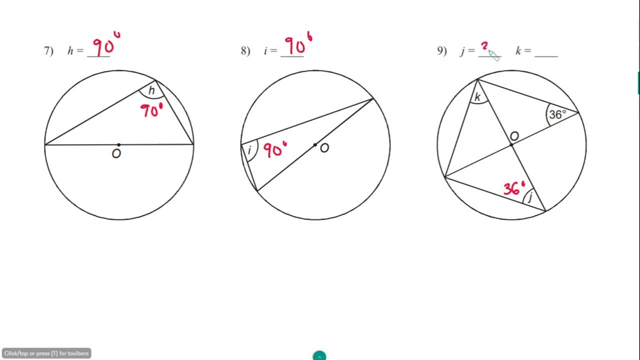 Okay, So I'm already on 36 degrees here. That's angle J, So that's 36 degrees, Okay, And to find angle K, I'm going to consider this triangle. Okay, And this is diameter passing through center O. 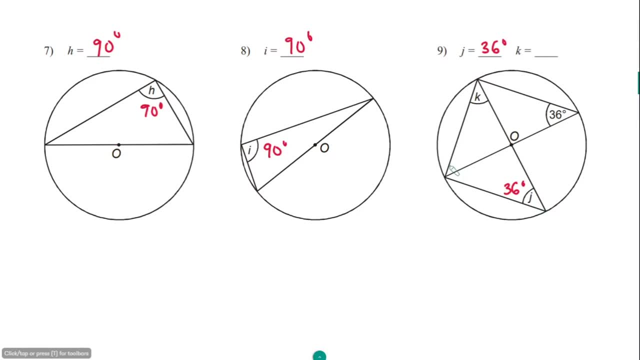 Okay. So this triangle, that means this angle is going to be 90 degree, definitely for sure. Okay, It's going to be 90 degree or half right degree, Okay. So if I add up this 90 and 36 and subtract from 180, I'm going to get angle for K. 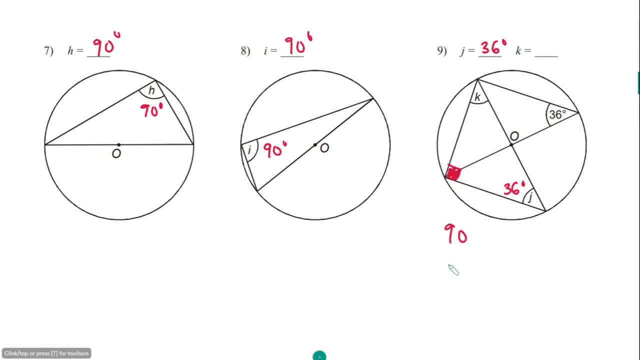 So I go straight by adding 90 degree and 36.. That's going to give me 126 degree And this I'm going to subtract from 180 to get K. So 180 degree subtract 126.. This is going to give me 54 degrees. 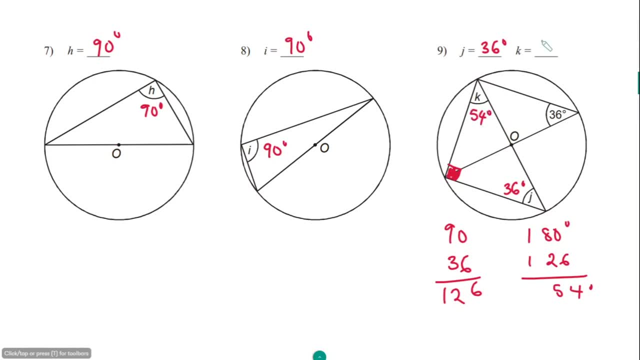 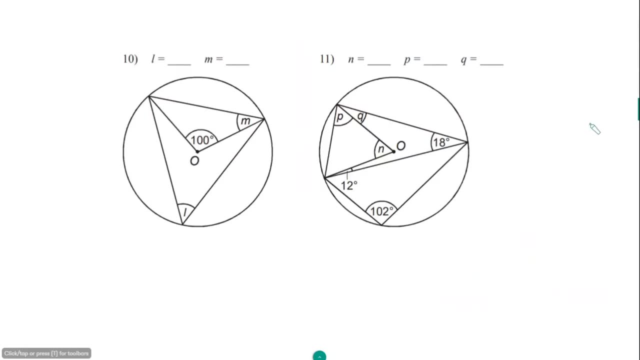 So angle K is going to be 54 degree. That was pretty easy, Right, All right. So let's move on to the next question, Question number 10.. We got our sub-circle problem here, Right, Good, Now we need to find angle L. Now, the angle made at the center here is already 100 degrees. 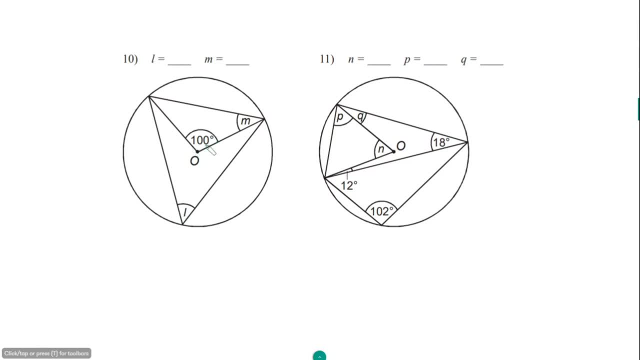 Add the circle of freedom, you have of it Okay, Because angle at the center is always twice the angle at the circle of freedom. So angle L definitely going to be 100 degree divided by 2. And that's going to be K. 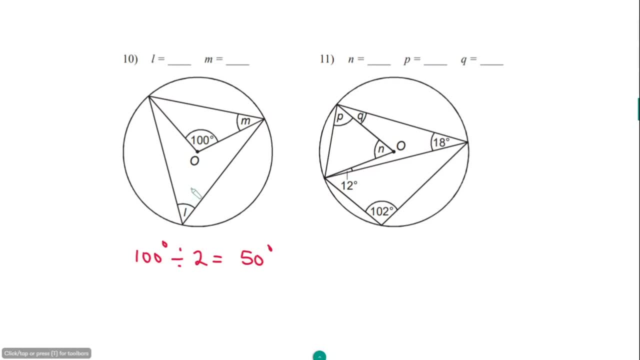 That's going to be 50 degree. So L is 50 degree And so put it up here 50 degree. Next we have to work out the angle M. Now, if you look at this question very well, you can find this at center O. 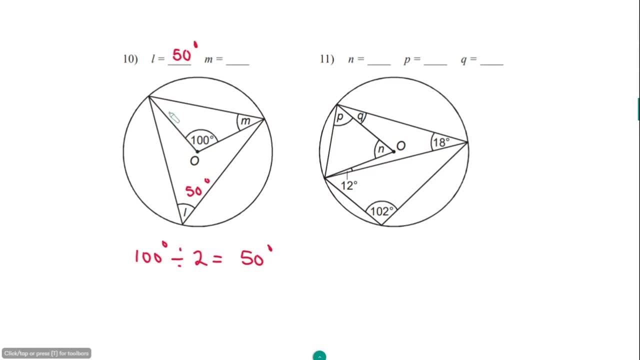 And with a radius here, another radius here. Okay, And equal. And if they're equal it means the base angles should also be equal. So here should also be angle M. Okay, Now I know the base angle should add up to. 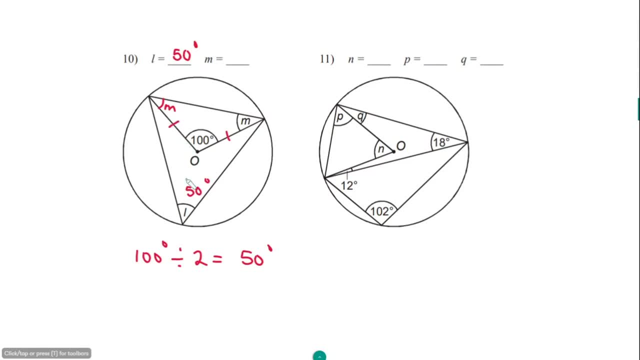 I mean the base angle should be equal for a facetious triangle. Okay, So to find angle M, I'm going to subtract, I'm going to do, Or I can do something. add M and M and add it to 100 to give 180. 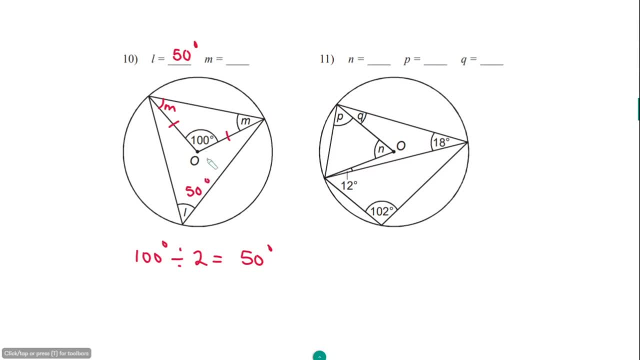 Right, Or for M, or you could just say 180 minus 100 and divide it by 2 to get one on each of angle M. Okay, But I'm going to use that method. I'm going to say 180 here. 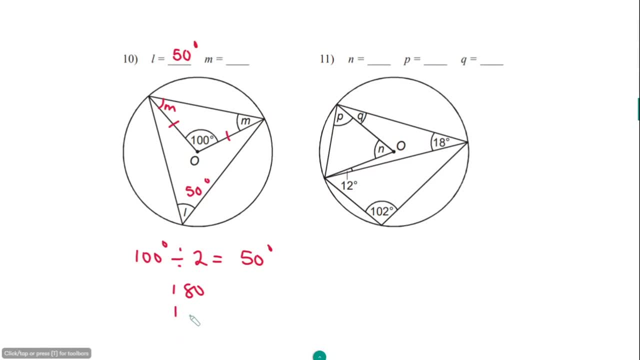 Subtract 100 degree And that's going to give me 80 degree. Okay, Now this 80 degree, I'm going to divide it into 2 to get each of the angle for M, We're going to be 40 degree. 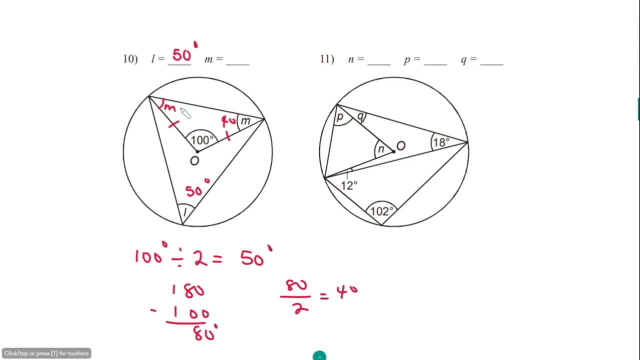 So here is 40 degree, M is 40 degree And here is going to be also be 40 degree. Okay, So M is 40 degree. So I come here, Right on here: 40 degree, Okay, All right, we come to question 11.. 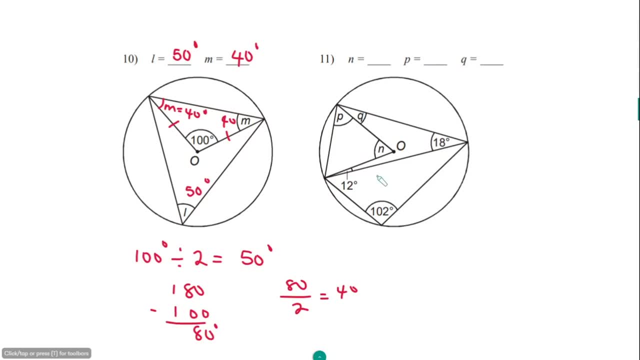 And we got some really complex problem here. But we can really do some working here. We need to find angle N, P and Q. Which one can we get first? Yeah, we can get N, Okay, Because angle at the center here is twice the angle of the second phrase here. 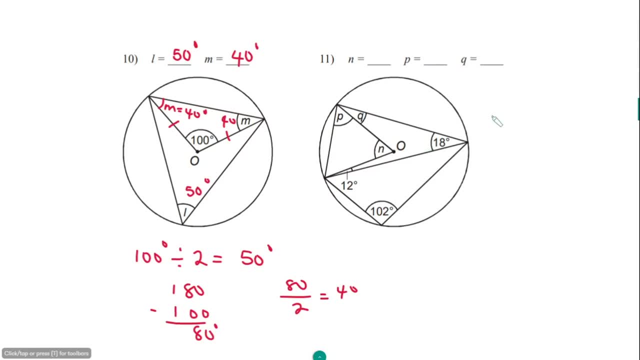 Okay, So N definitely going to be 18 times 2.. And I'm going to give you 36 degree, So N is going to be 36 degree. Okay, 0.1.. Easy one. Next we get angle P. 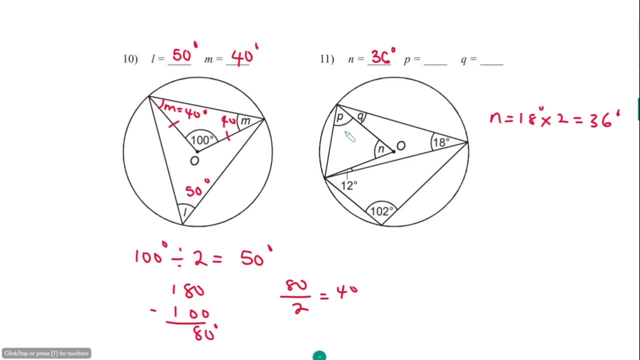 Now, how do we get angle P? Now this is angle P here. Well, that's very easy, Because see this from here, from center O down. here is the radius, And same from center O here to other, here is also radius. 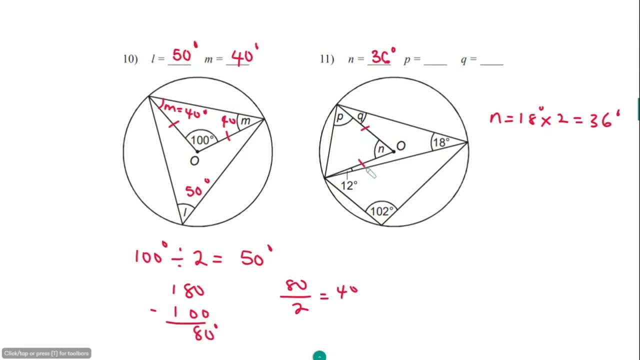 So that means this length here should be equal to this length here And that's going to be an accessible triangle, Okay, And that means this base angle here should also be angle P. Okay, I already know N is 36 degree. All I need to do is to subtract to find angle P is to subtract this angle 36 from 180.. 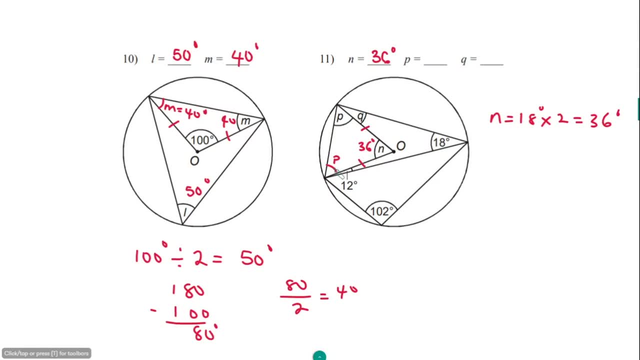 And then halve it to find individual angles for P And this other angle here, virtual P. Okay, So what I'm going to do first is to say 180 degree minus 36 degree, This is going to give 4.. 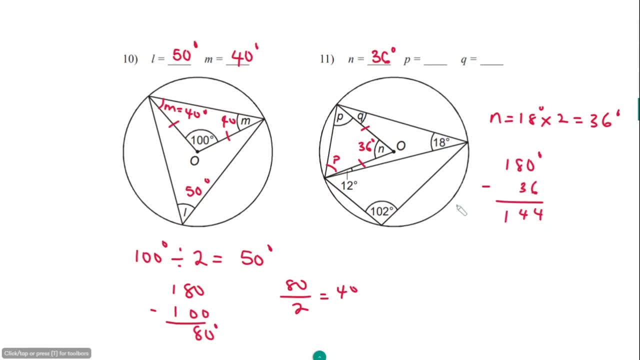 5.. Okay, 4.. 104 degrees. Okay, Then, to find each angle P here, and also this virtual angle P, I'm going to divide 144, divided by 2. And that's going to give me 72 degree. 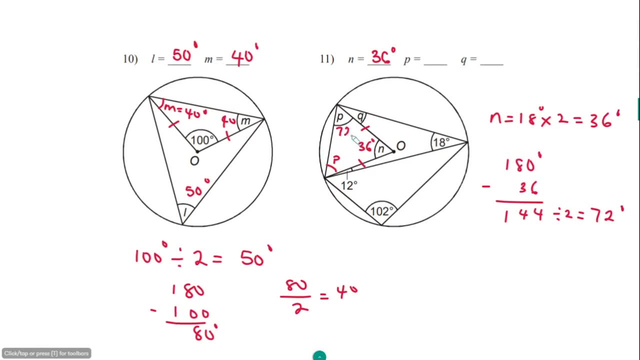 So that means angle P is going to be 72 here degree And also here this angle P here is going to be also 72 degree. So I come here right: Angle P is 72 degree And next we need to find angle Q. 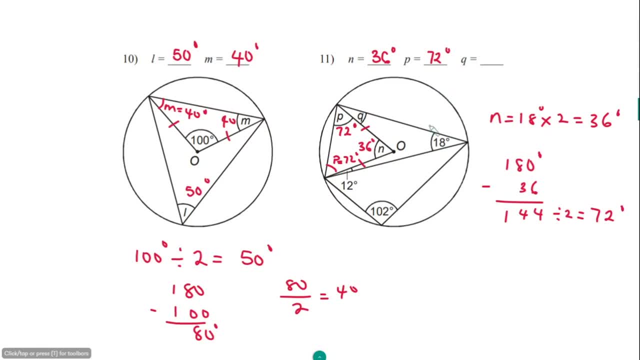 Well, there are a number of ways you can find angle, angle Q. One way you could do this is, I mean, a very fast way to do that is I already know that P, Q, just add up these two angles here. 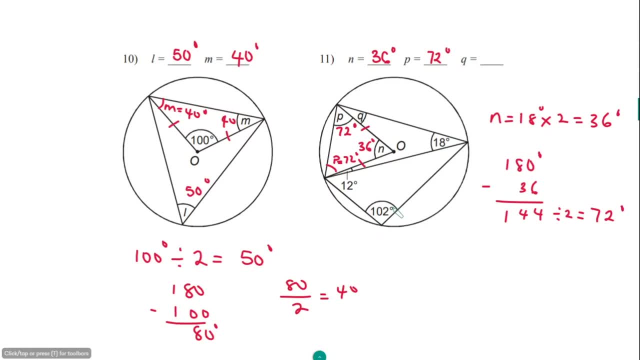 Okay, And that should always be equal to 180.. I mean, these two angles, P and Q, and 102, add up to 180,. right, Because it's cyclic quadrilateral. Okay, All right. So what I'm going to do here, I'm going to say P plus Q. 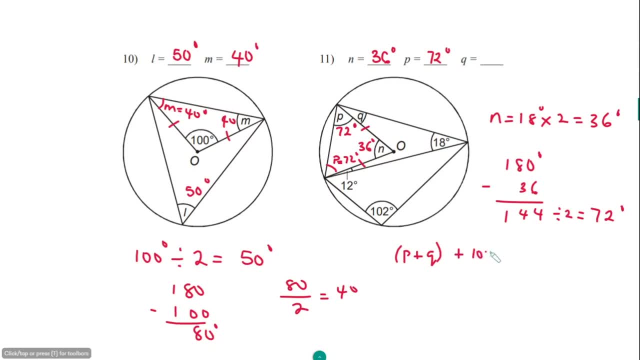 Okay, This angle. Add up to 102 degree, That's going to be 180 degree. Why? Because this is the opposite angle of a cyclic quadrilateral. Because we have the quadrilateral here already in a second. Now I already know angle P to be 72.. 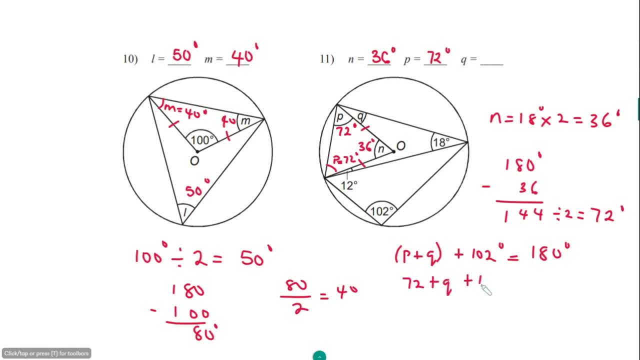 So I have 72 plus Q, plus 102 is equal to 180 degree. Now if I add up 72 plus 102, I'm going to have 174 degree And this goes to 180.. And to get angle Q, you subtract: 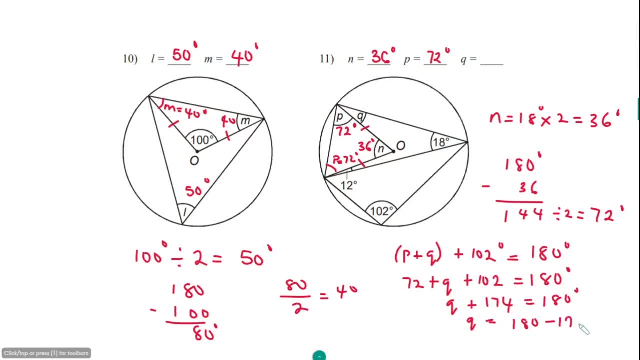 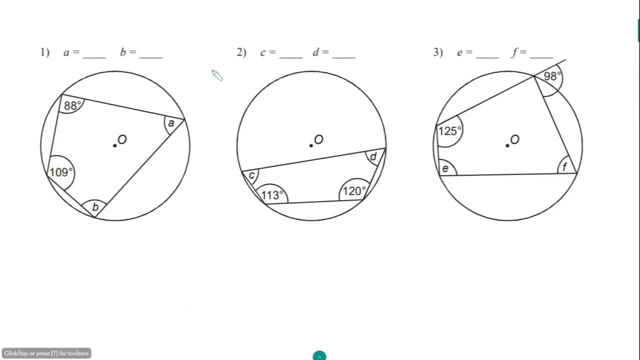 I do subtract 174 from 180. And that's going to give you 6 degree. Okay, I'll give you 6 degree. So that means angle Q is actually 6 degree. Okay, Now in this question we need to find the various angles: A, B, C, D, E and F. 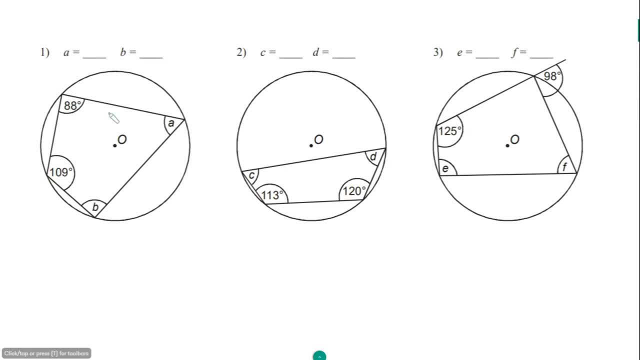 But first angle A. Now, this is a cyclic quadrilateral. Okay, In a cycle, Okay, And we need to find the angle A. The opposite angle of a cyclic quadrilateral always add up to 180.. So to find angle B, I'm going to find the angle A. 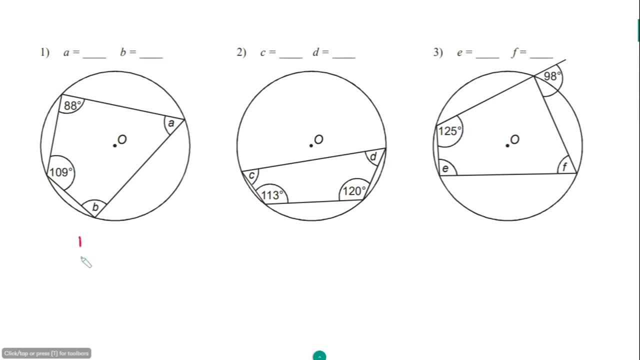 Let me get angle A first. Okay, Angle A is going to be 180 degree. I'll subtract 109.. Okay, This is going to give me a subtract. It's going to be 1.. Okay, 7.. So 71 degree angle. 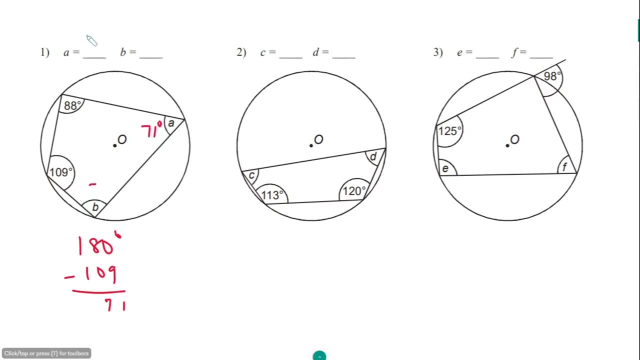 Angle A is 71 degree. Okay, A is 71 degree. To work out angle B, I'm going to subtract 188 from 180.. Okay, And that's going to be 29.. Correct, So angle B is going to be 92 degree. 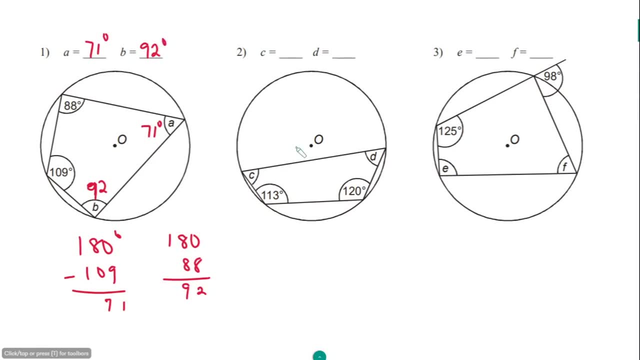 So B is 92 degree. All right For this. another cyclic quadrilateral: the opposite angles always add up to 180.. Okay, So angle C is definitely going to be 180.. C and I want to add up 180.. 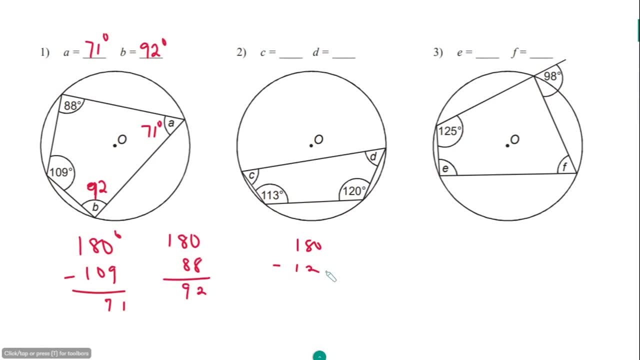 So to get C, 180 minus 120.. And that's going to be 60.. So angle C is 60 degree. Okay, So C is 60 degree. For D, the same thing We'll do: 180.. 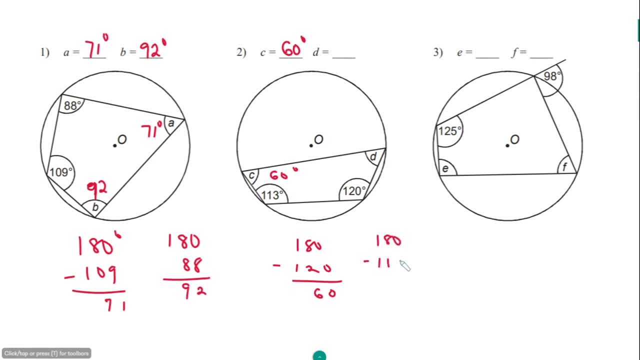 Subtract 103.. 413 rather 7.. Mmm 67.. So it's going to be 67 degree. So D is 67 degree. If you add them up, you're going to see they're going to have 180 degree. 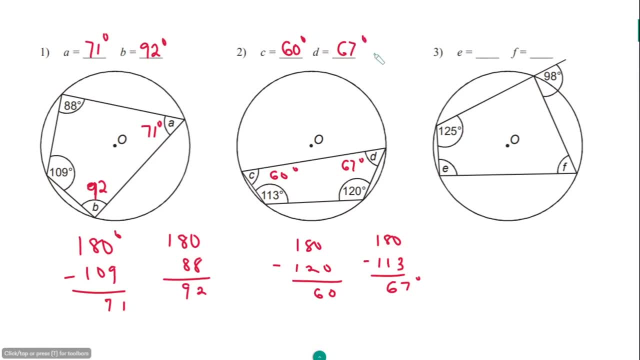 So this is going to be 67 degree. And now we come to question three. Now we need to find angle E. Okay, All right, So find angle E. well, you can consider that this line here is a straight line and the standard angle is 98.. 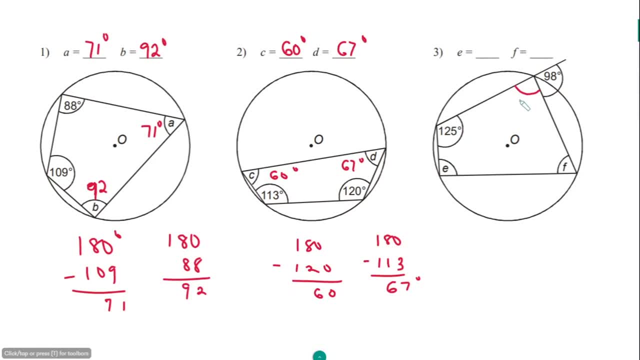 now, to find this angle here, i'm going to do 180 minus 98. okay, let me do 180 minus 98. it's going to be two. i'm going to be 82 also, and i should write, um, um good, 82, 82.. so they're going to be 82 degree. 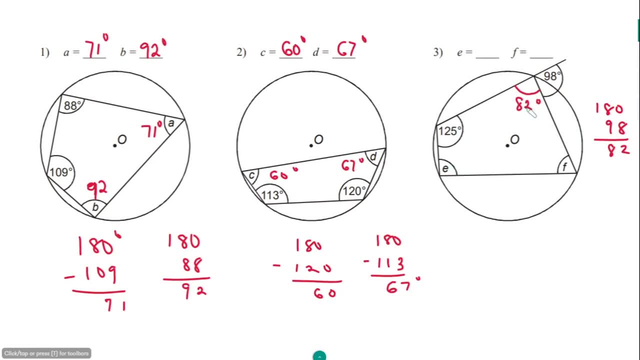 all right, and to find the angle, e, this angle, add up e and they should give you 180.. so to find the angle here, i'm going to subtract these two from 180.. so let's do 180, subtract 82. okay, you have eight here and they could have, uh, nine, so 98. so this angle is going. 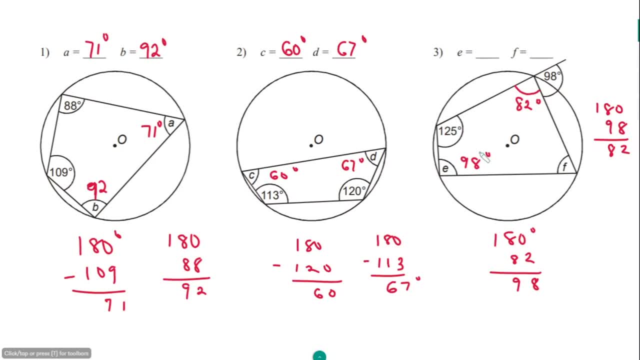 to be 98 degree. so here's 98 degree to find angle f. well, we've got opposite angle, second quadrature, add up to 180.. so i'm going to find and find angle f. i'm going to subtract this value 1 to 5 from 180. 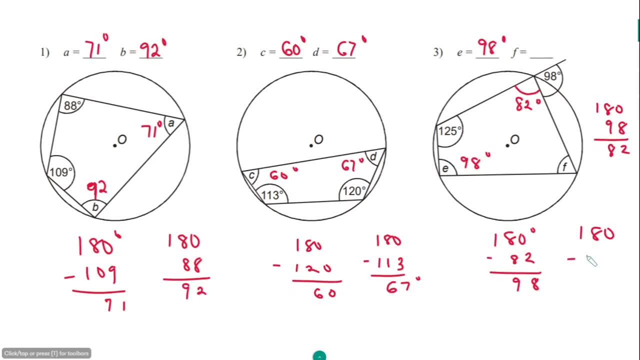 so 180 degree, subtract um 125, that's going to be 55 degree. so angle f is going to be 55 degree. okay, now, just out of interest. if you add up this opposite angle, you'll find the one is add up to 180. the same for this and the same for this also. okay, all right, so let's move on. 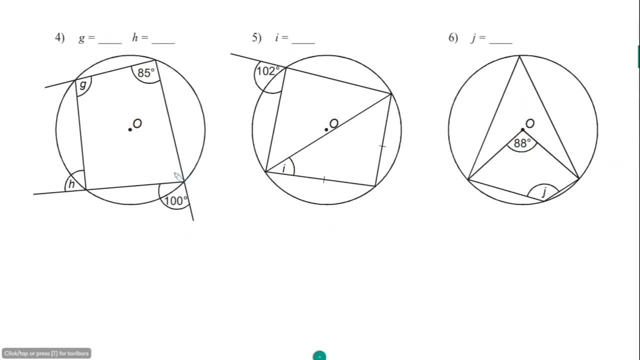 to the next question. all right, uh, we need to find out with gh. okay, here to find angle g or angle h, but let me say angle um, let's say angle, hey, g first. but i know you have a straight line here. here's 100 degrees, here can be a hundred. so eight out of 180, around 80. so you're going to. 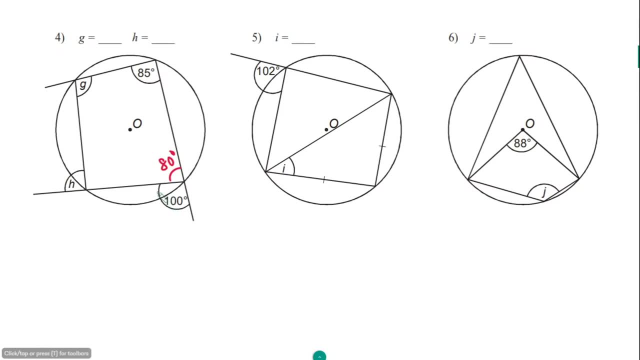 be 80 degrees. okay, because i'm going to straight line- is 180.. okay, so if he has 80, this angle, both angles should be equals- g and 80 should add up to 180.. so that's, g is going to be 100 degree. 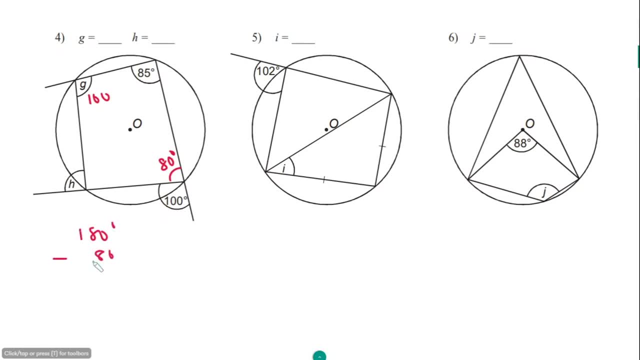 i'm going to do 180 degrees minus 80.. of course, it's going to be 100 degrees. that's how i got this 100 degrees here. so i'm going to use 100 degree for angle h. well, one thing i can tell is: 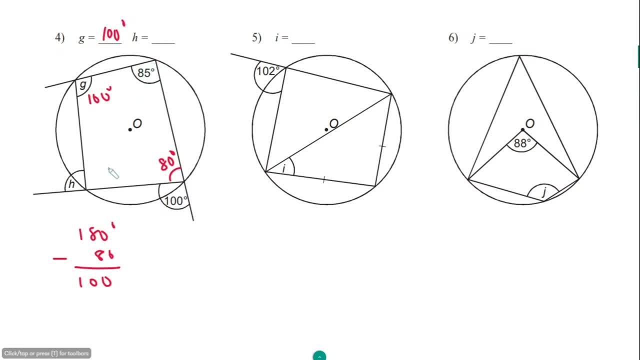 that, um, this angle here is going to be to find this angle here. i'm going to subtract it from 180, so 180 minus 85, uh, five, so here's my seven. so so much in the possible answer here. 70 minus eight, um, that's going to give you. 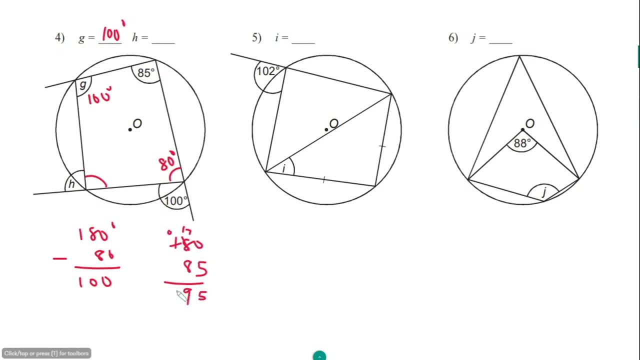 nine. okay, of course here is zero anyway, so 95. so it is going to be 95 degree, okay. and to find angle, h- remember i'm going to straight line- is 180. so h is going to be 180, um 180 minus 95 again. 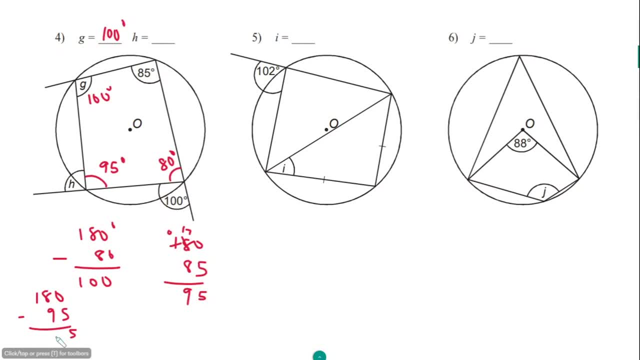 you have five subtract um and you have 85, okay, so angle h is going to be 85 degree, so h is 85 degree. and then we come up here. now we need to find angle i here, this angle i um. now we've got a triangle here already. we know. 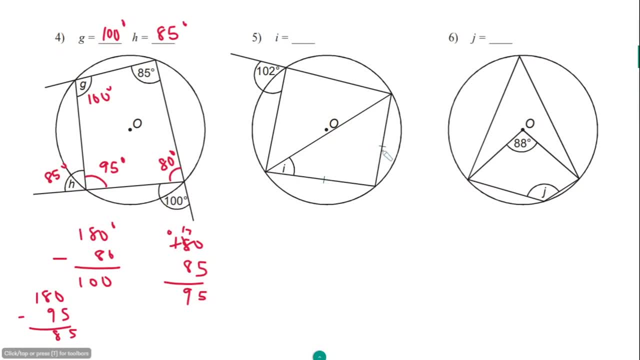 uh, that this length here is equal to this length here. that means the angle i here should also be equal to the angle i here. okay, but let's continue. but again, you have a straight line here and this angle here, like this, two angles should add up to 180.. so if here's one on two, 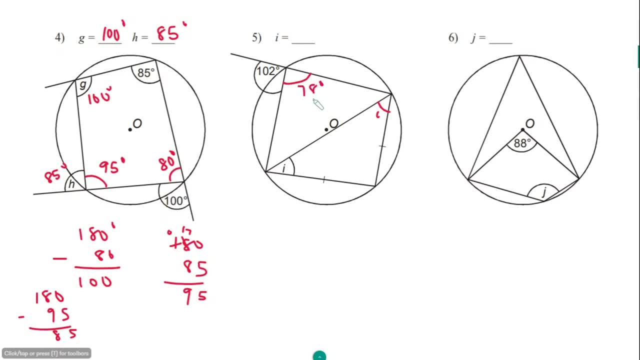 this is. i'm going to be 78, okay, 78. and how do i know it's 78? all i need to do is to subtract 102 from 180 and of course, that's going to give you 78. okay, so, if here's something, 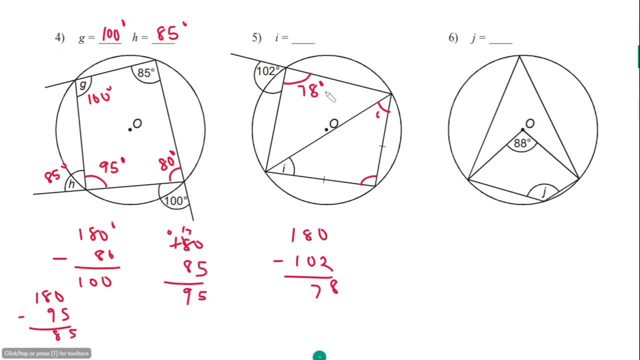 in a square. the two things what i'm conjugating here are the triangle양 and the two angles. so now what i'd do is i'll do 180.. okay, so now you will measure it and this is the perfect angle. so simultaneously, okay, oh, i should tell you that you can do this with the awful angle. 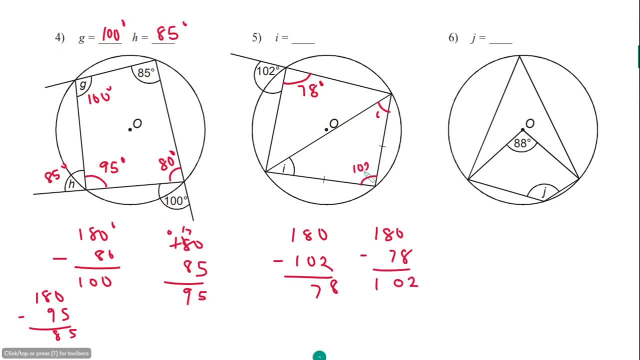 this angle j i. i've only done up to 180. okay, see, fill the triangle. this j also should be 70 degree. okay, equal. all I need to do is to subtract 1 or 2 from 180 and the result I get divided by 2 to get individual angles for the base angles here on the triangle. 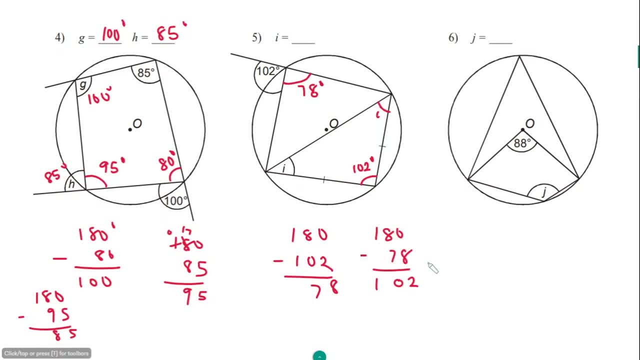 okay. so what I'm going to do here, I'm going to do: I'm going to do something like 180, I'll subtract 102, which will give me 78. now this angle 78, I want to divide it by 2 to get individual angle here. so I'm going to do 78 divided by 2. 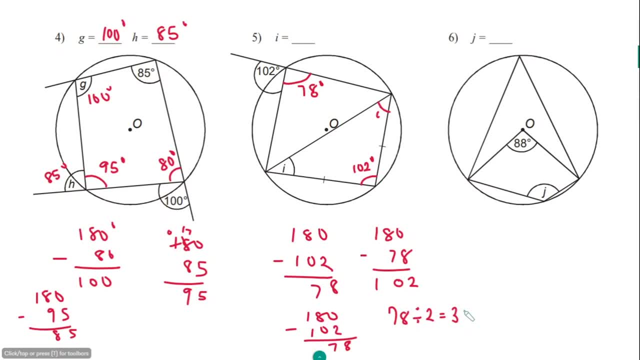 that's going to give me 39 degree, so angle I is going to be 39 degree. okay, also, here is 39 degree. now, if you add up this triangle, you're going to find out. of this angles, you're gonna find out. I'm giving on 80 degrees, so angle I is 39. 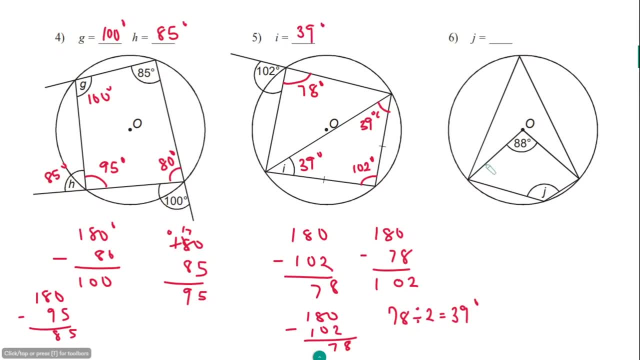 degree. and then we come to question six and we got a kind of a drawing here and we need to find a good chain. one of these you could do is the number of ways you could do. you could find this reference angle here and then divide by two to get a good J. okay, all you could. 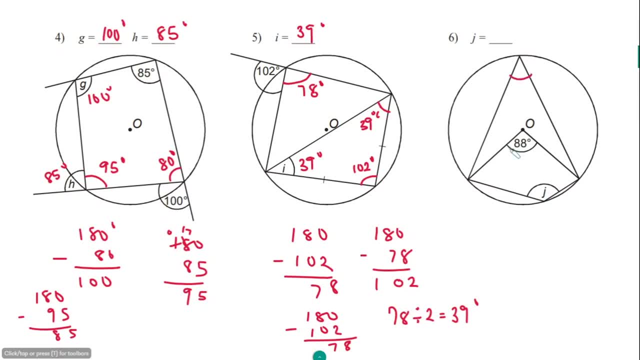 just think of this time we here to be 44 because I was sent out, it's gonna be twice the angle circumference. so if he is 88, definitely here has been 44, okay, and then they can now consider that this angle here- and I'm with J- add up to 180. 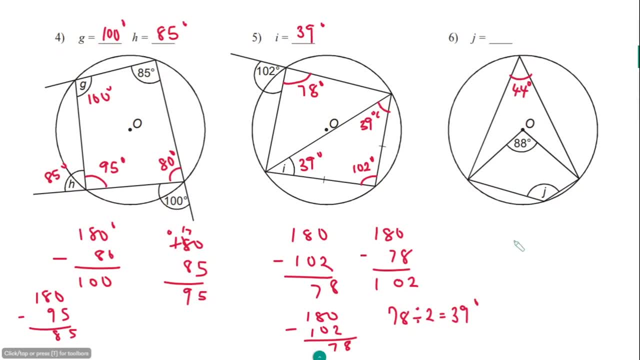 because you have a cycling for the latter. okay, so that means I'm gonna do 180 minus forty four six. it will give me 36 degrees. so I'm gonna be a hundred and thirty six degree, because if you add up G and this angle here, I'm gonna give you 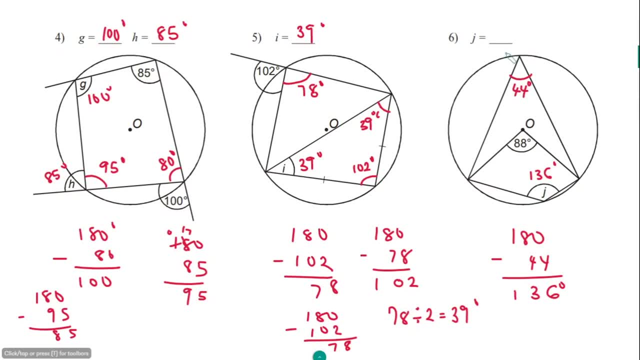 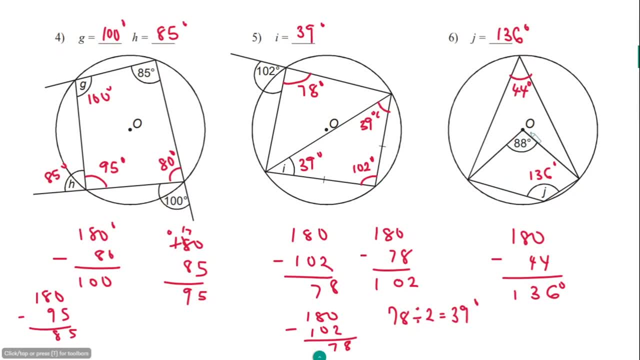 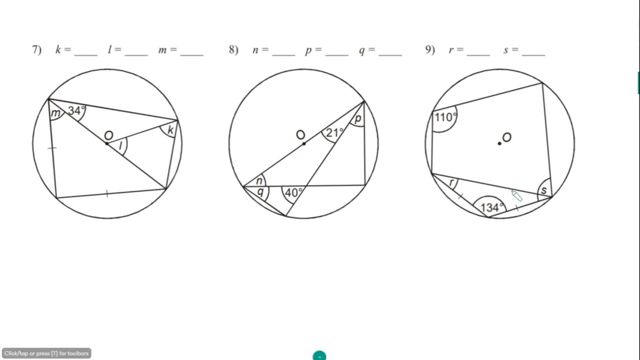 okay, like I said, you could find this angle here, but somebody 360 and then whatever I get you also. divide by two, you get a good J. all right, okay, so let's move on to next. we got some real difficult question here. we know those may have problem trying to figure out how to solve this problem by the pro. 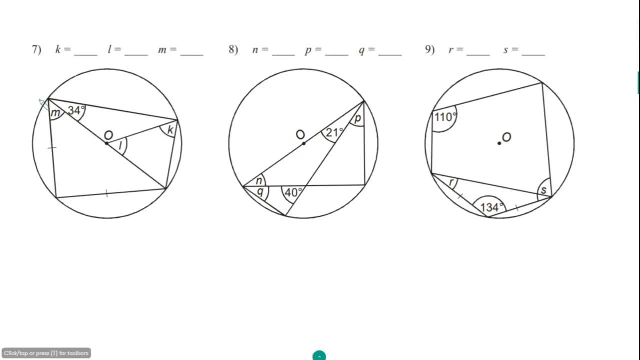 let's try it here. we got the center, okay with sent a diameter here. we said, oh all right, and we know this length here is equals to this length here, and I also have the radius here, another radius, meaning that this length here should be equals to this length here. all right, okay so to find angle M, but because we're 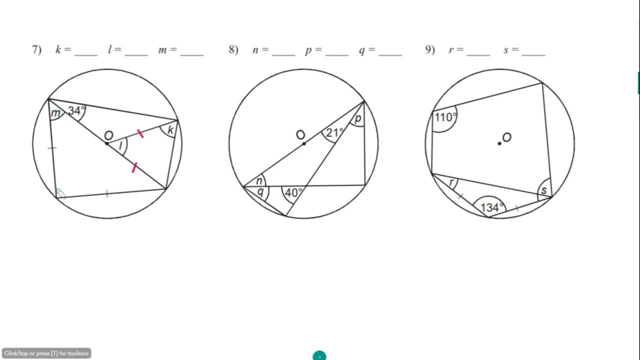 anything that is in diameter and this angle semicircle. I mean. that means that this angle, I just will be 90 degree. okay, all right. and to get this angle M, all I need to do is subtract 90 from 180- whatever I get, and a half it. okay, so I. 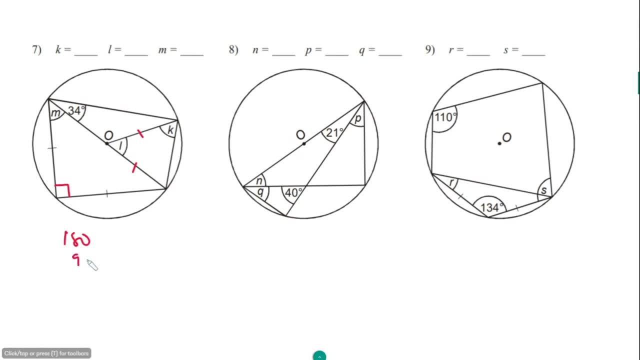 will have 180 here, minus 90, because it's angry here. definitely equal to M, okay, all right. so if I subtract is gonna be 90, okay, and then, if I could have this, you gonna have this 90 divided by 2, we have 45, so angle M gonna be 45 here, and also. 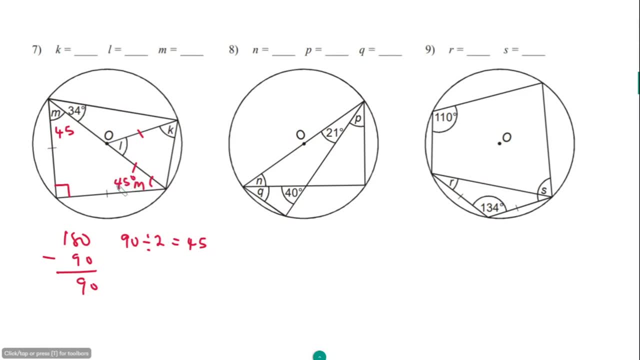 here gonna be 45. okay, if I really want to write it down, okay, it mean the same thing: 45 degrees here, 45 degree also. yeah. so angle M is going to be 45 degree, okay. next we need to put out angle K or L. now. one thing you can consider here is that 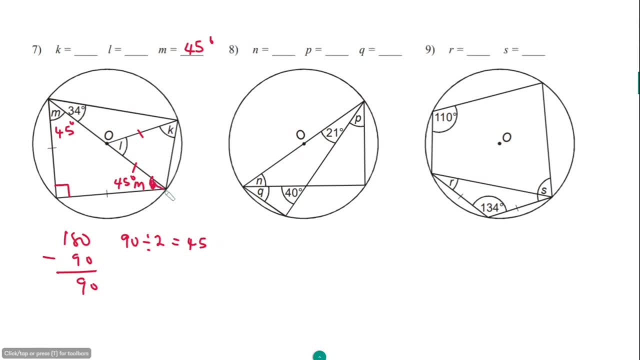 okay, I'm gonna try to see what I'm gonna do. let me try to shade here. okay, let me see what I'm gonna do here, to find either: well, if this is angle K, here also has to be angle K, right? yeah, it makes some sense, it will say so. 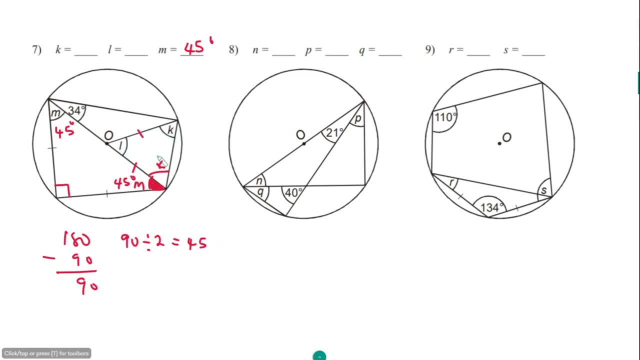 because this length is because it's length, and so the base angle of triangle should be always be equal. so we need to find angle K or L. alright, one thing you can consider which is very easy: if here is an angle. here is 90 second, friends. I need to find an angle at the center. all you need to do is multiply by. 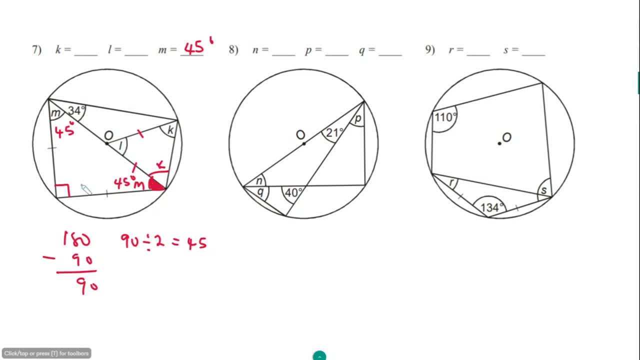 two, right, okay. so let's say angle K here is 80, except for gonna be 180. okay, alright, but I don't think that's gonna work. what I can do here is just trying to figure out what I'm gonna do here. okay, good, these two angle here. okay, these two angle here. 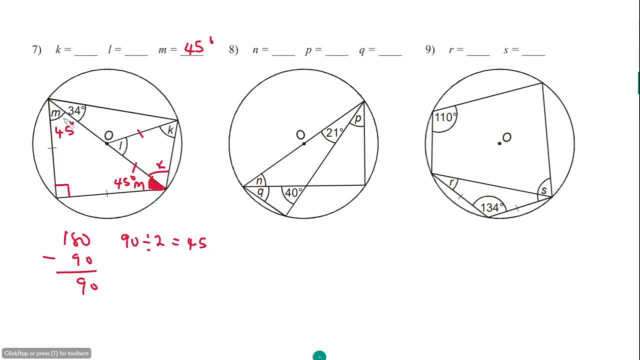 should equals to this two angle here, because I mean they should add up to 180. remember angle opposite angle, exactly quadrilateral, or is 80, 180, it's this here- and add this anguish given on 80. so what I'm going to do is to say I'll add: 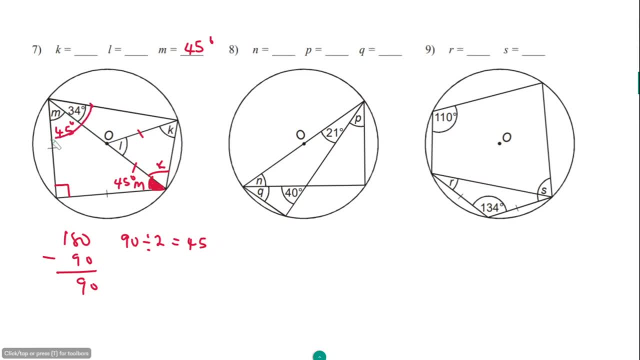 up this, to angle this, to agree here, it's just for the 45 and 34. okay, and add up to this only here, which is 45 plus K, okay, should give me 180 degree, okay. so if I add this value, these two here, I'm gonna have. we'll have 79 degree plus 45. 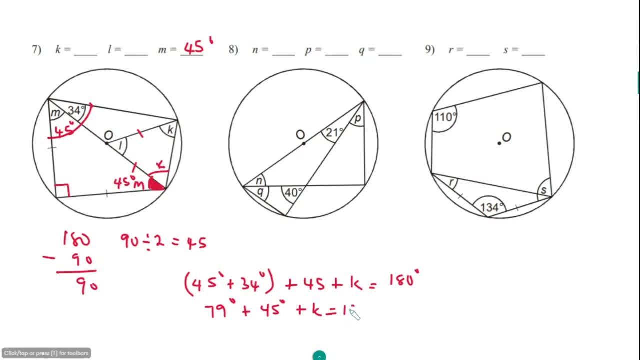 plus K is equals to 180 degree and if I add this, I'm gonna have 4 here. 124 plus K is equals to 180 degree. so get uncle K. okay, it's definitely going to be on 18 minus 124 and that's gonna give me 56 degree. so I'm good and case with the 6 degree. 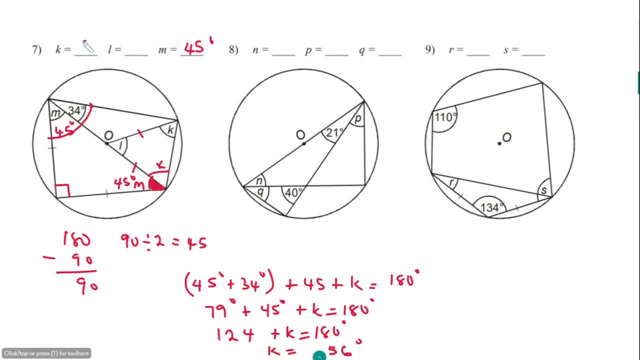 okay, so in case gonna be 56 degree. okay, all right. so to get angle L, that these two angle K, K and L should add up to 180. so if this is plus 56 subtracted from 180, to get angle L. so I'm gonna do 56, 56 degree at 56 degree I'm gonna give. 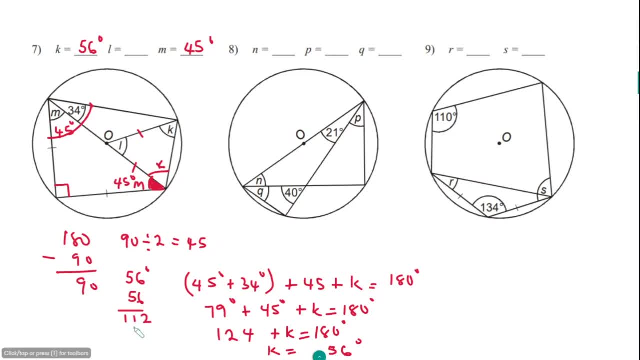 me 112 and we'll surprise that from 180. so 180 subtract 112, okay, that's gonna give you 68. so I'm gonna be 68 degree, all right. that was pretty, very difficult, okay, all right. so let's move on to the next question. eight, eight- we need to work out- and P and Q, you can see. 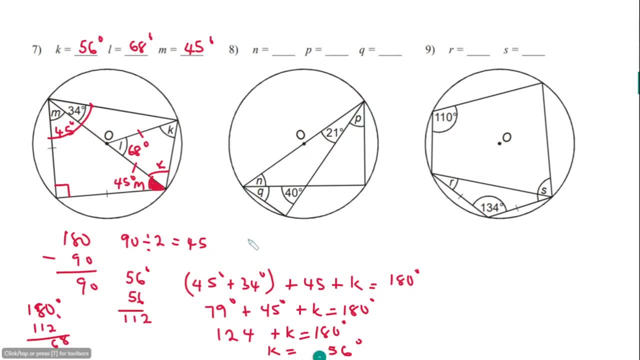 the center hole. okay, the diameter, all right, what you know, hidden before two degrees. okay, you know why? because you got vertical opposite angle, all right. so so how do you find n, P, n or Q? all right, but definitely persist, since this is a diameter and how I'll go. 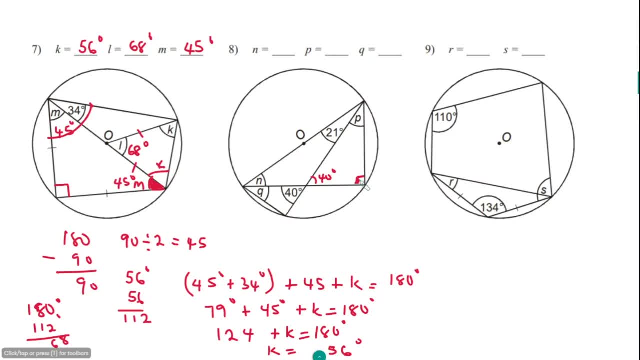 in the same circle, this angle, then it will be 90 degree. okay, so I'm going to shit it. I mean 90 degree, all right. so to find out the piece, very easy, just consider this triangle here. okay, so I have 90 plus 40 and 90 plus 40 here. 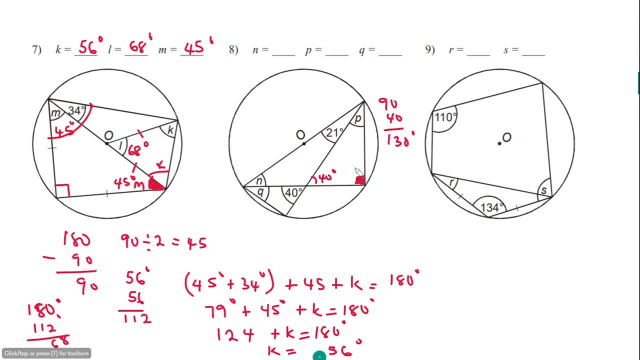 130 and separate from 180. so 180 subtract 130 and then 50 degree. so angle P is 50 degree, single piece, 50 degree here. all right. so we need to find angle n and P. now that you can consider, you got a straight line here. so if this: 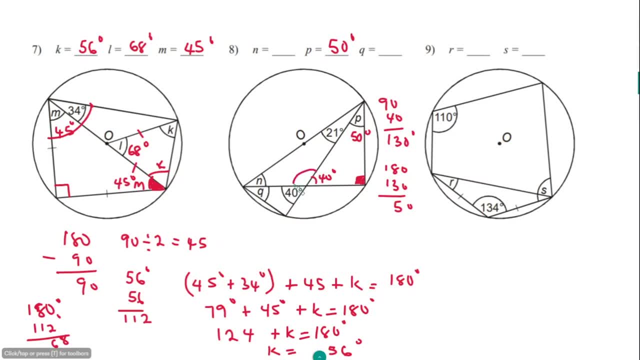 if here is 40 degree, then we can also find it here. there's gonna be okay. we have 140, right, because these two angles should add up to 180, all right. so if I study this triangle here, I have 140 plus 21, plus n should be add up to 180. so 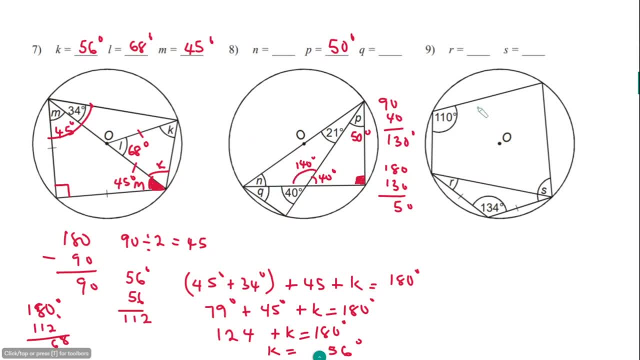 what I'm gonna do to find n is add up 140 plus 21. okay, I'm gonna do it here. 140- okay, that's gonna be too far. okay, let me take that away from there. let me do the work in here somewhere here. so 140 plus. 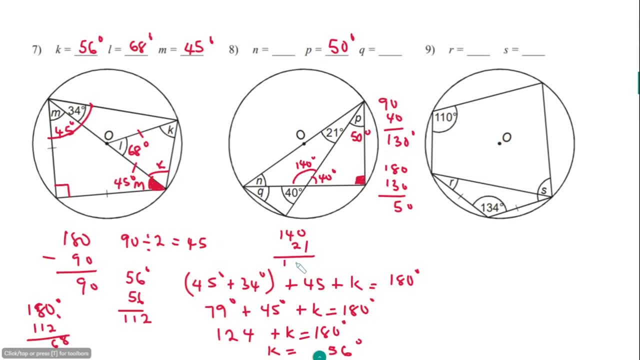 21, that's 161. okay, I'm gonna subtract it from 180, so 180 minus 161, and that's gonna give me 19 degrees. so n is gonna be 19 degrees and it's 19 degree, all right. so two down the many one, which is Q, to find Q, what we may consider. 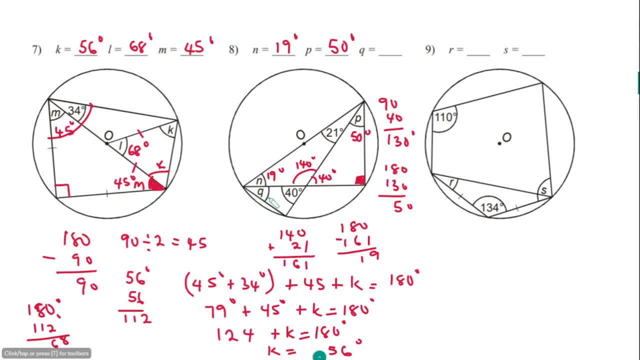 here is okay. the angle Q is also in the same segment with P. so if P is 50, Q has to also be 50 degree. okay, that's very easy to spot. all right, so we come to one last question, number nine. we need to find angle R as t. 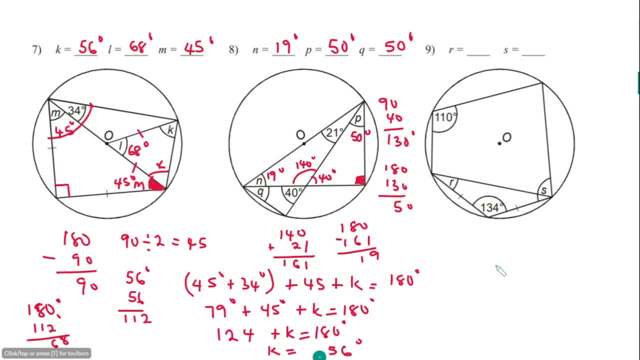 9xx. all right, so one more question, number nine: we need to find angle R as t, angle R as t. now we know that we have, uh, two lines marked okay, meaning that they are the same. so definitely this angle here is going to be angle r, really okay. so what we can do, we know, if here is 134, we can. 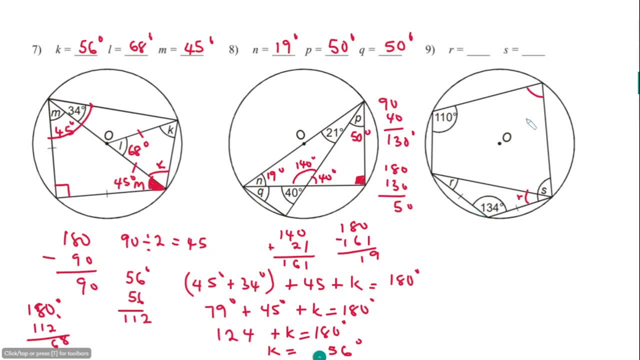 also find here, because the sum of the sum up to 180. okay, it's opposite angle. the second quadrilateral is 180, so i'm going for 180 minus 134. here there's going to be: um, this is going to be 46, so this angle here is going to be 46 degree, okay. 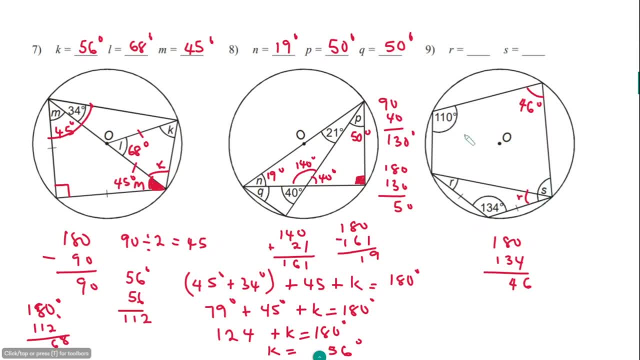 and if i to find angle x, well, i can also think that this angle here and angle s add up to 180. angles opposite angle with second equilateral add up to 180. okay, so angle s definitely going to be 180 minus 110, okay, that's 70. so angle x here is actually 70 degree. the full angle here is: 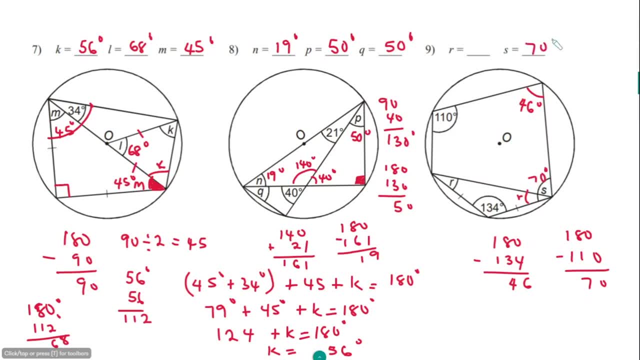 70 degree. okay, so s is 70 degree, and then i need to find angle r. well, that's very easy. like i said, these are under here. this angle i'm going to shade, that's what i'm referring. okay, i'm going to do is i'm going to add angle r plus angle r plus 34. wanted to add 34, give 180 degrees. so if i add up, 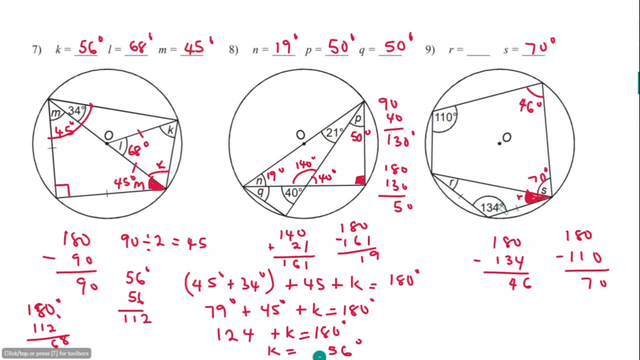 uh, what i'm going to add. 180 is what one easy to get our r is to subtract 134, 180, okay, and that's uh six um 46, and then divided by two to get the individual angles for r here and the other. so 46 divided by two, this is going to give 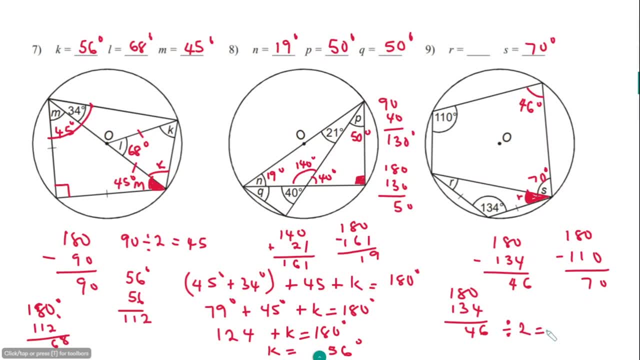 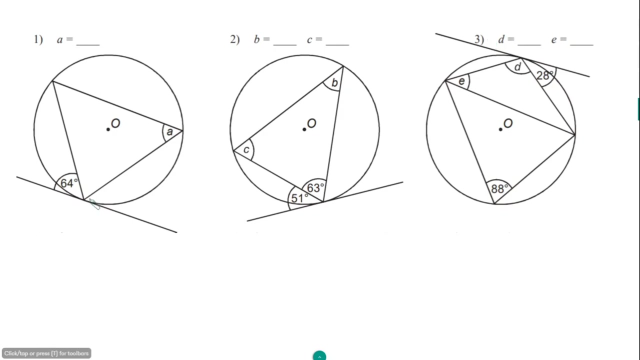 me: oh, it's gonna be 23 degrees, so R is gonna be 23 degrees. Wow, that was real, real tough, okay, so let's move on to the next question, all right, so we we need to work out the angle. a. now, this is all tiny segments, dollars equal, so it's a. 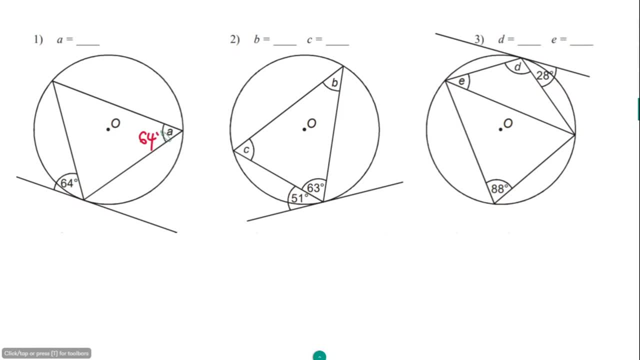 here is 64, here has also be 64 degree. very easy, okay, alternate segments are equal and the same for here. if here is 51 and would be has to be 51, alternate segments are equal. okay. and then to find, we see, you can cause, you can think of these three angles, you add up 180, I'm gonna triangle. 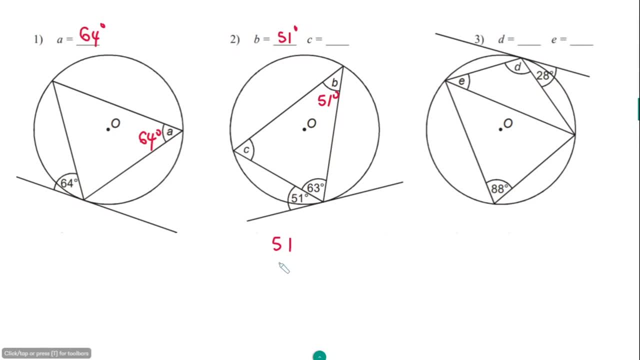 so I'm gonna add up 51 and 63. 51 add 63, that's gonna give me 114. and to get it and see a little, subtract this: 180. this is gonna give me 66 degrees. so I see, is 66 degree? all right, ok, so now we move to the third question. so we need to find 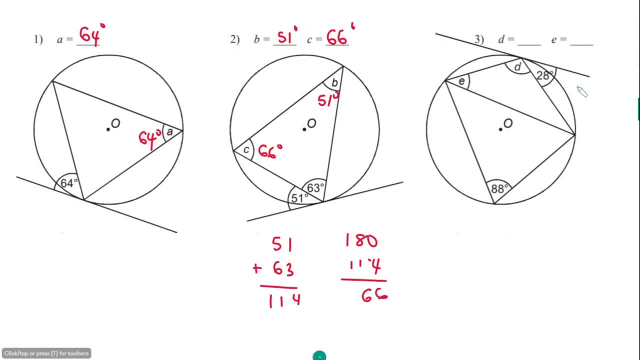 angle d and e. we have the tangent drawn here and good, excited poly lateral here, and these two, angle d and 88, should add up to 180. opposite angles of a cyclic collider also add up to 180.. so then i've got angle d. all i need to do is to subtract. 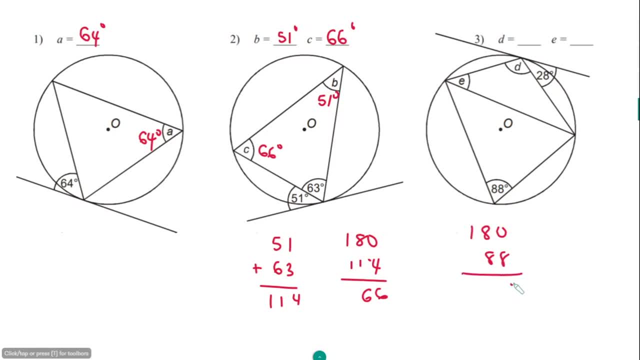 uh 88 from 180 degrees i'm gonna have um 92. okay, yeah, 92. so angle d is 92 degree. okay, so these 92 degree. next we have to work out the angle uh e. well, it depends on what you're looking at, but if you kind of turn this round you 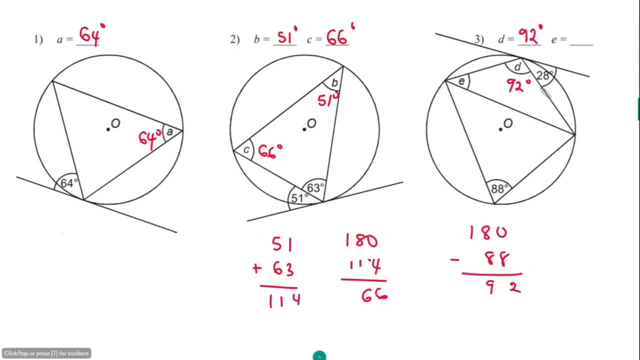 you'll immediately see that this angle here is alternate segment to e. i mean, that's it. so he's gonna be 28 degree because alternate angle are equal. all right, that's, that's very easy, right? good, all right, so let's move on to the next question. 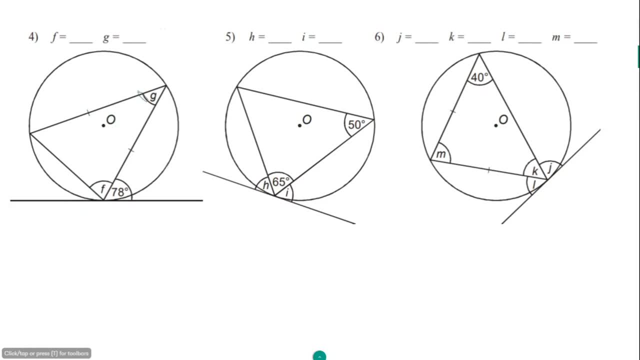 we got a cycle and a triangle inside here and the tangent and this triangle, the length here is equals to the length here. okay, i mean, if base, if he has f here, there will also be angle f, because the base angle of an associate triangle are always equal. okay, so if, uh, here's 78 angle f definitely. 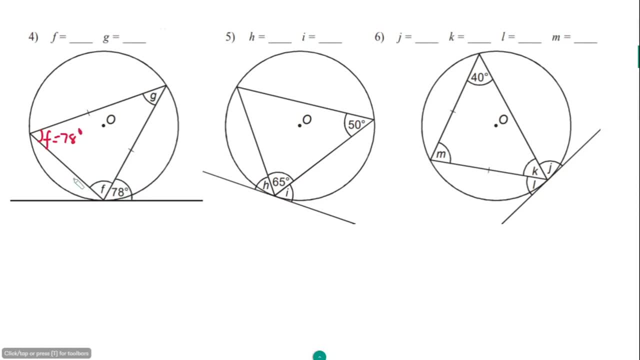 78 because the atomic segment angles are always equal. so f is going to be 78 degree. to find angle g i need to add up these three angles. to add up to give me 180 and the final g- well here is something- eight. anyway, we know that because the base angle are equal. so out of 78 and 78. 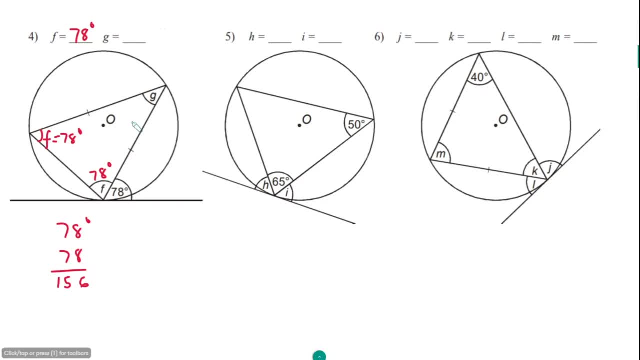 i'm going to have 156.. to find angle g, i'm going to subtract this from 180, because we have some of angle triangles: 180. so 180 subtract 156. uh, you have um 24. so i'm going angle g is going to be 24 degree. okay, yeah, 24 degrees, somewhere around 24 degree here. 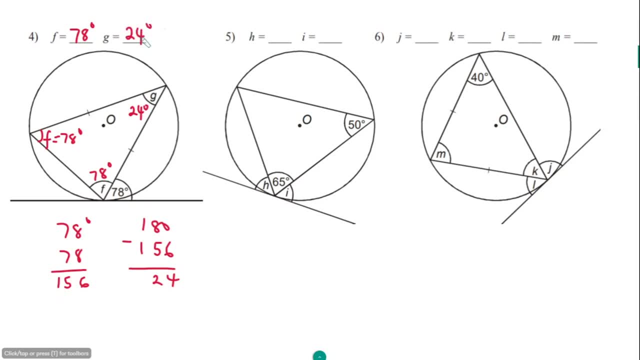 so here it will be 24 degree. we're making good progress, right. okay, now for number five, we need to find angle h and i, hmm, all right, but first i know this and, uh, in this angle i definitely could be the same angle here. okay, so if i know this angle, that's. 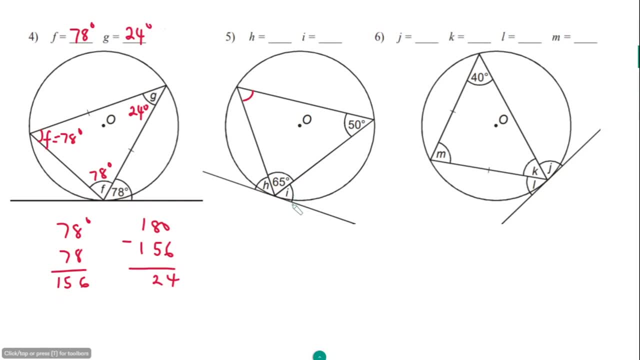 a good angle. i, because we have alternate segment, all right, but one okay. one way we can do this is, uh, to think of the sum of angle triangles: 180. so if you have 65 and 50 here, we're going to be angry here in the triangle. so i'm going to add 65 and 50 and that's going to be 115 to find this. 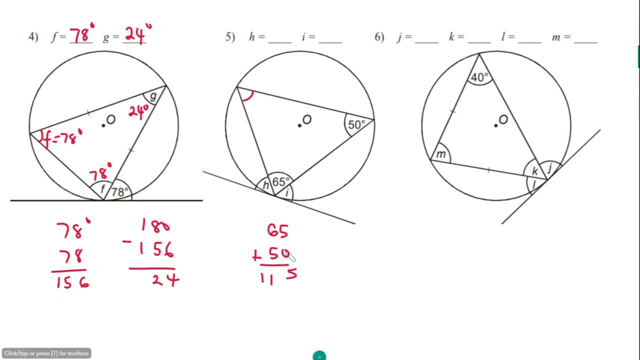 angle here. i'm going to subtract this from 180. okay, so i'm going to subtract this from 180. okay, now, if i subtract this, i'm going to have 65. so this angle is going to be 65 degree and angle i is, uh, alternate segment to angle i and the always angle is already the same. 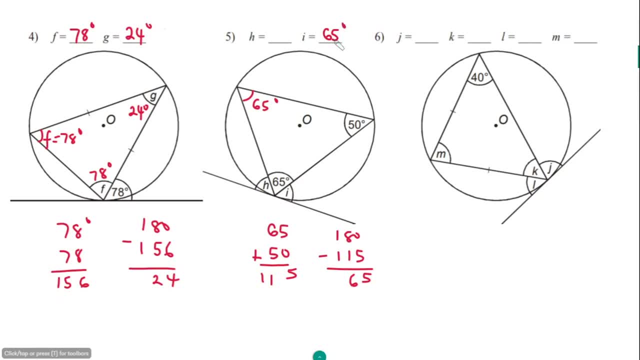 so angle i is going to be 65 degree already. we already know that angle- this angle, 50 degrees, is alternate segment to angle h, so h is going to be 50 degrees as well. okay, all right, so we move on six. now we got some angles jklm that we need to find. i don't have this triangle here. it. 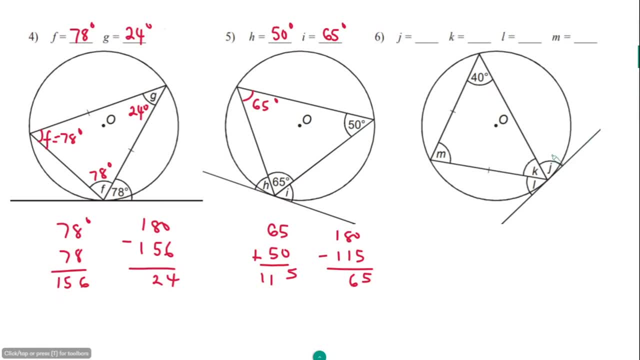 enclipsed with the cycle and then you got a tangent here. now what do we know about an assessment triangle? that is that they are always the base angles are always the same. so if here is 40, because we have this right here, okay, so here's 40. the base angle k also has to be 40 degree. 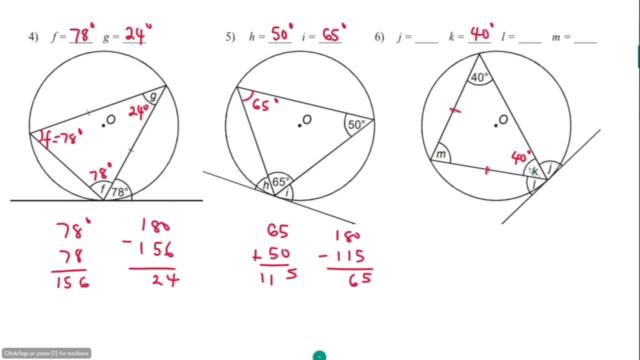 so k is 40 degree, okay, and uh, and i know that this angle, is it l? yep, i've got l is alternate segment to angle 40 also, so here's going to also be 40, okay, so that's going to be 40.. auto is going to equal. 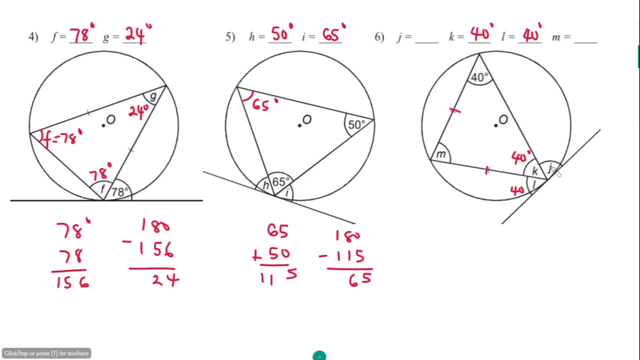 all, right, now we've got a straight line here. okay, now this three angles should add up to 180. okay, so if here is 40, 40 to get here, j is going to be 100. okay, because you see they should add up to 180. okay, all right, let me just show you the working 40. 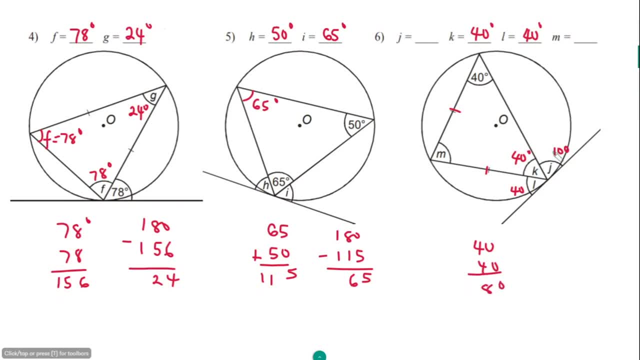 plus 40, that's going to give you 80 degree. right, and remember, these three angles add up to 180, because angle straight line is 180.. so i'm going to subtract this 80 from 180 and that's going to give me 100 degree. okay, so angle j is 100 degree and this angle is also. 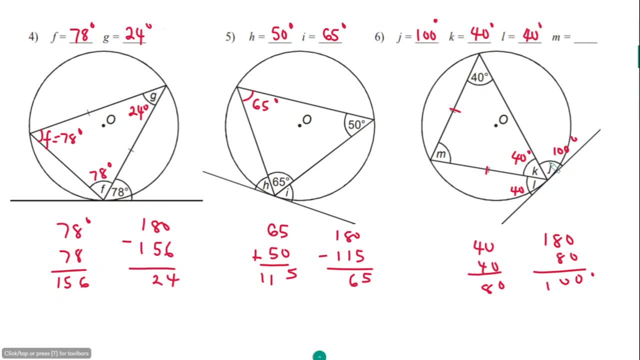 be uh, alternate segment of a segment to m. they have this. they should have the same angle, so it's going to be 100 degree as well. okay, all right now. you might have noticed that you could go to angle m another way by looking at, thinking that you have a triangle here. okay, these three angles. 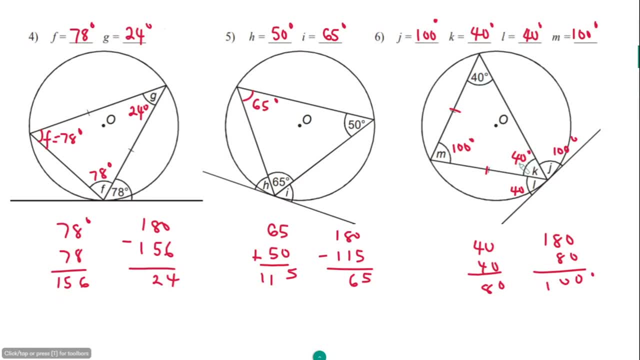 should add up to 180.. so if here is 40, 40, just 80 to be 180 in the triangle, uh, subtract 80 from 180, you're going to have 100. okay, so that's another way to you could want to solve that okay. 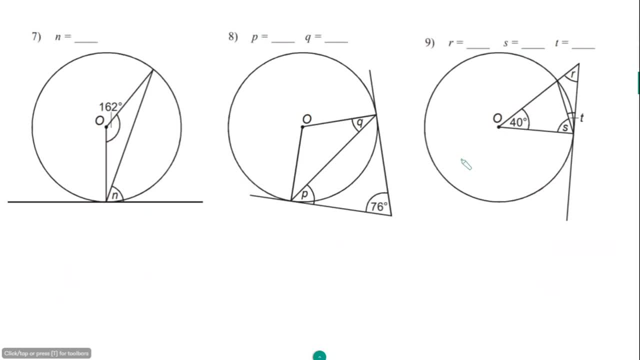 all right, uh, so we move on to question n. here we got: uh, you see, notice that we have a segment here and a radius, okay, meaning that this whole angle here must be 90 degrees. but first, let's not go through that route first, okay, okay, first thing, we got a radius. another radius here. 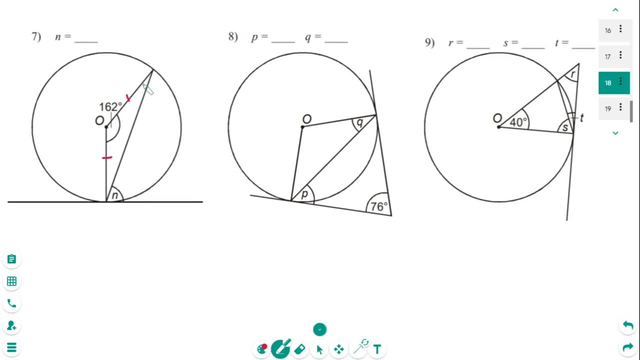 that means the length here should be because of this length, okay, and the angle here should always be also be equal to the angle here. okay, this angle here, the base number here, should also be equal to the base angle here. so to find each of the base angle, all i need to just subtract these from 180. 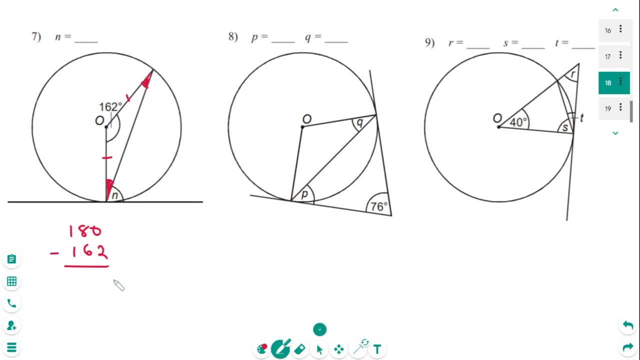 that's 180 minus 162. if you subtract that, that will give you 18. okay, so to find each of the base angle here divides its angle 18.. okay, okay, so to find each of the base angle here divides its angle auf 180.. 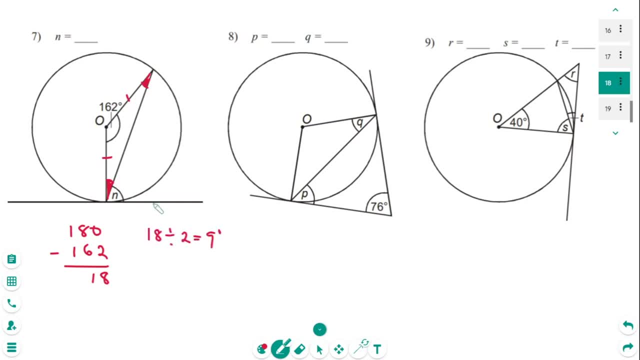 by 2 and that's going to give you 9 degrees. so each year is 9 degree also, here's only 9 degree. okay, and I always also know, as I said at the beginning, but yeah, this is, this is radius. I have a diameter, I mean a tangent, now the radius. 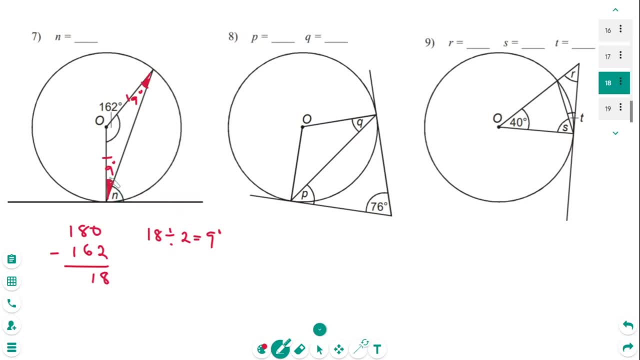 means that a tangent at 90 degrees. so this how under here is 90 degree. so if yes, night, and it will be 90, take away 9 and that's going to be um 81 degree. so go, and it's going to be 81 degree. that's pretty easy, right? and then we'll go to. 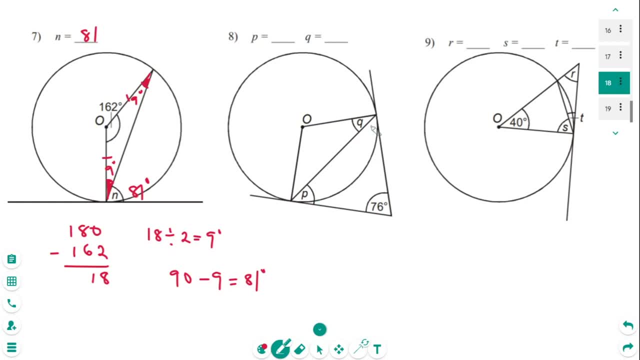 question number 8: now we need to find angle P and angle Q. now we have this: good, I'm having a tangent here drawn here and telling John here, and then we have a tangent here drawn here and then we have here also meaning that this length here should be equal to this length here. so 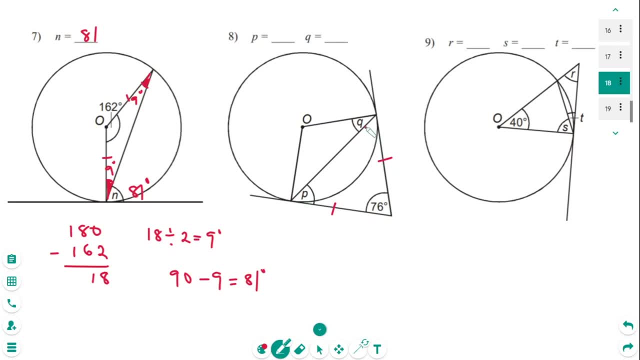 if you look at this triangle here, here gonna be a good P also because they're gonna be the same. so to find angle P: okay, you subtract 76 from 180, okay, that's gonna be 104. so to find each angle here on the base of triangle. 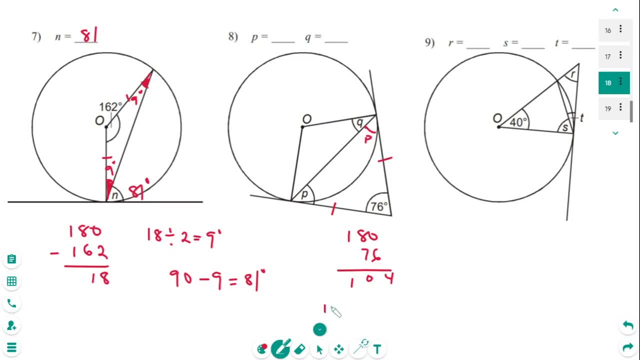 divided value: okay, 104 divided by 2, that will be 52 degrees. so each angle here is 52 degree. here also 52 degree. okay, okay, there's gonna be 52 degree also. so we know, P is 52 degrees. so right after the 2 degree here: okay, now we need to find angle Q. now. 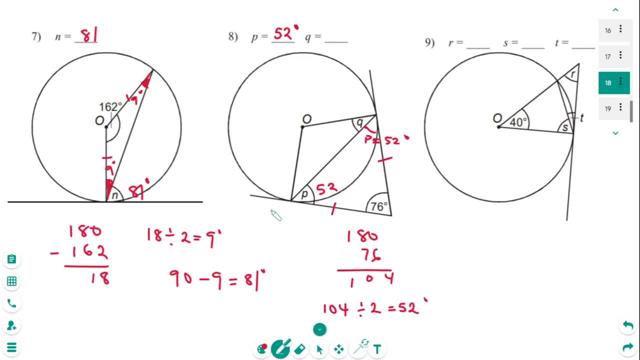 to do that. one thing we can think of is, since this is center and this is a radius, this length should also be equal to this radius here. so here has to also be angle Q also right, my station, all right. so, but what we know is this: together Q all. 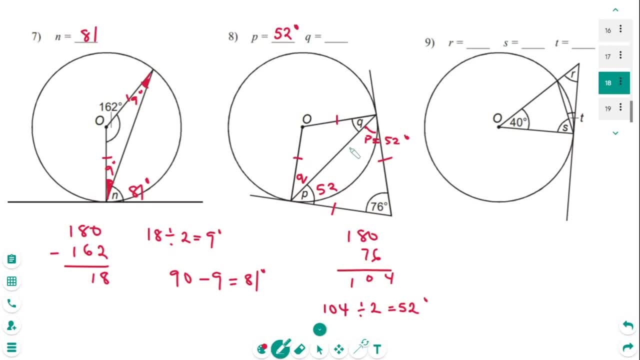 right, remember, we could do something like: yes, 52, here's 52. okay, I'm just thinking how I'm gonna walk this out. okay, all right, all right. okay. also, how soon that this is. this is a radius. okay, they have a tangent. also, this whole angle has to be 90 degrees. every smart one, okay, 90, okay, remember, a radius means. 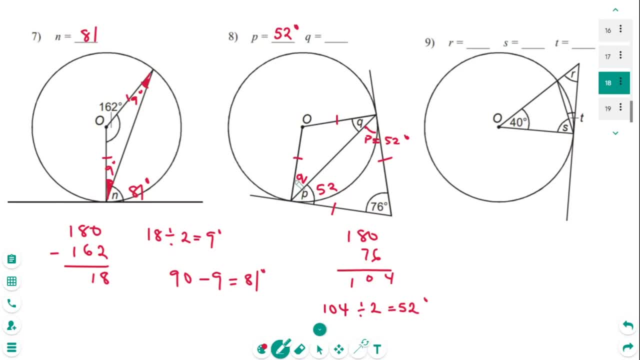 a tangent at 90 degrees all the time. so this angle has the whole angle. here you can see when my key, my pen, is moving. the whole angle here is gonna be 90. may not angle P and Q: adoption: 19. so the fight and Q: you subtract 52 from 90. 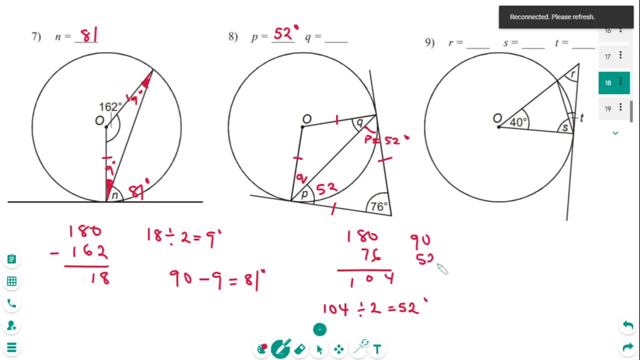 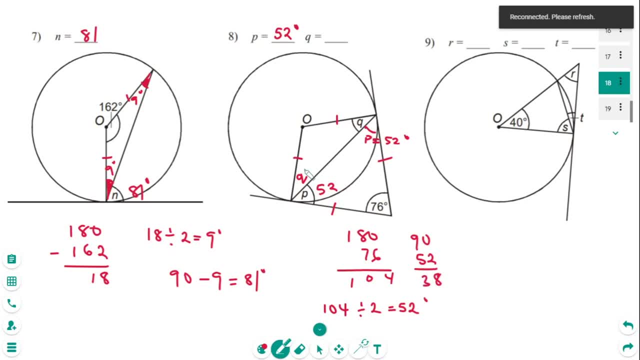 to 90 minus 52. that's gonna to 90 minus 52. that's gonna give you 38 degrees. so angle Q you're gonna be give you 38 degrees. so angle Q you're gonna be give you 38 degrees. so angle Q you're gonna be 30, 8 degree. so the Q is 30: 8 degree. 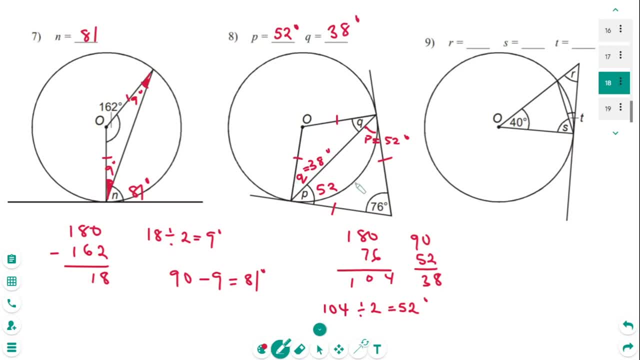 30, 8 degree, so the Q is 30, 8 degree: 30, 8 degree, so the Q is 30, 8 degree. that was very smart, right, good? and let's, that was very smart, right, good. and let's that was very smart, right, good. and let's come to question number nine. go ready to. 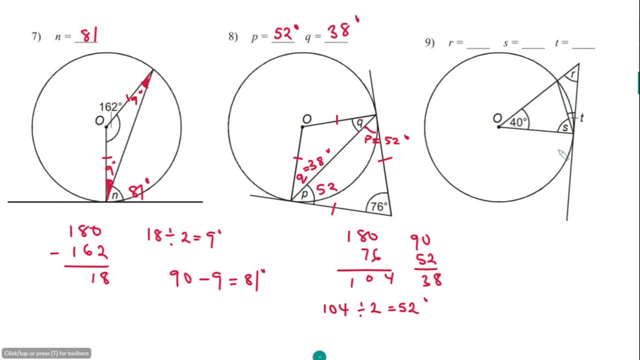 come to question number nine. go ready. to come to question number nine. go ready to find angle RS and T. okay, find angle RS and T, okay, And we have the center, and then we got a radius and we have a tangent And we know the radius makes an angle of 90 degrees with a tangent. so I have this angle s plus t definitely has to be 90 degrees, right. 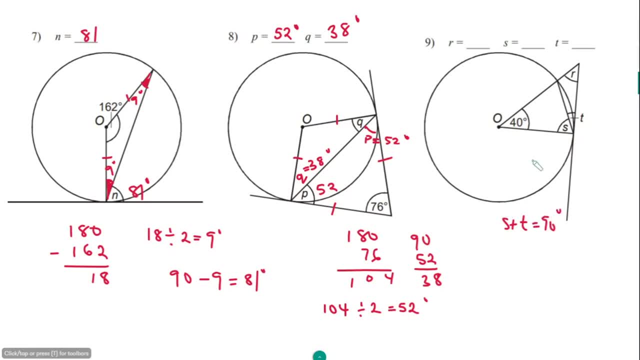 Okay, that's it for sure. And because this is a radius, okay, if I come in from the center, and also here this angle 2 is going to have to be angle s also okay. So to find angle s, all I need to do now is: this triangle should give me 180, angle triangle. so I need to do is to subtract 40 from 180, so 180 minus 40, and that's 140. 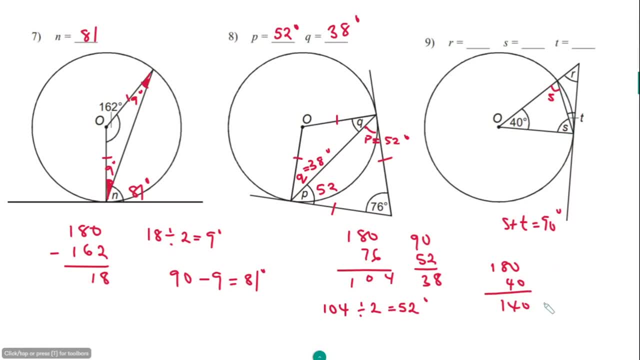 So to find angle s, each of the angle s here, I'm going to divide it by 2, so 140 divided by 2, that's going to be 70 degrees. So angle s is 70 degrees here. okay, 70 degrees. let me write it very well. so angle s is going to be also 70 degrees, but I don't have to rewrite it, okay. 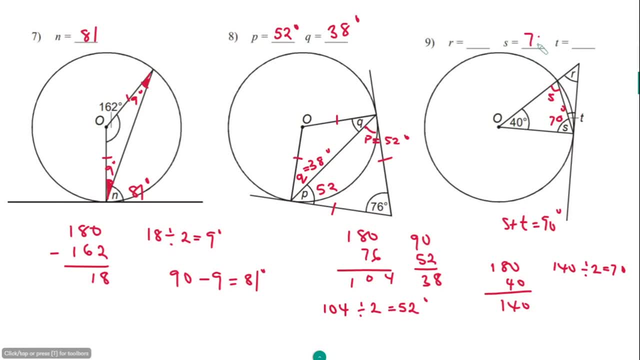 Angle s is going to be 70 degrees And remember we said s plus t, this angle 2, angle s is going to be 90, so if s is 70, t is going to be 90. So angle t is going to be 20, because 90 minus 70 is 20, so angle t is going to be 20 degrees. 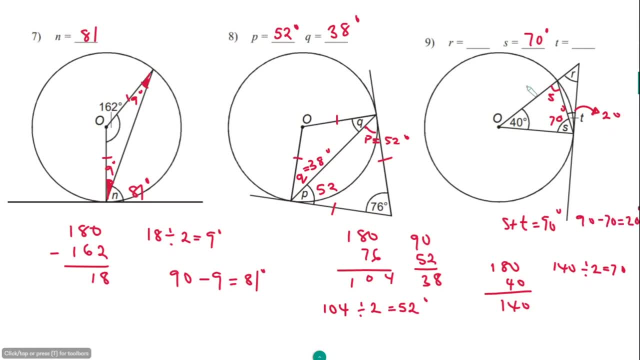 So that's 90 minus 70, and that's 20 degrees. So angle t is 20 degrees. Now to find angle r, you can consider this full triangle, okay, And remember the angle sum of a triangle add up to 180.. 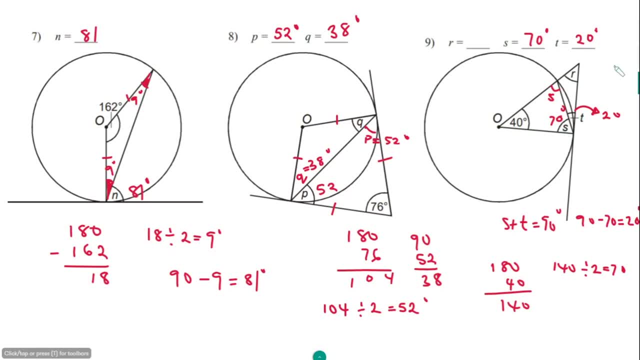 And you'll have your total 90 plus 40,. 90 plus 40,, that's going to be 130.. And to find angle r, okay, I'm going to subtract from 180, so I have 180 minus 130, okay. 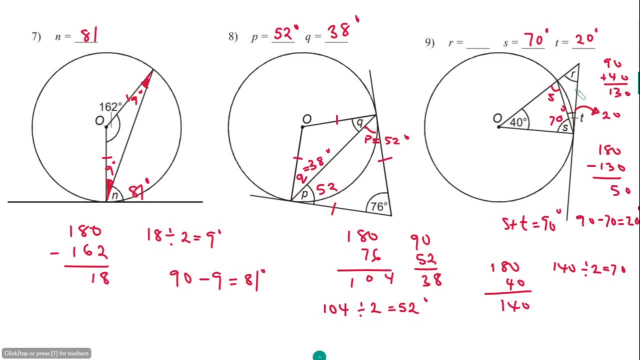 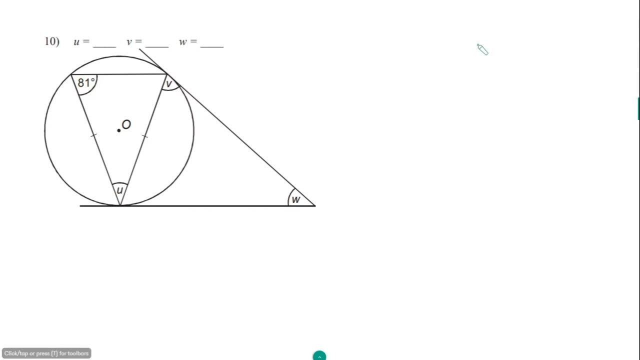 And that's going to be 50 degrees, so angle r is going to be 50 degrees. That was really really hectic. Okay, so we come to the last question, number 10.. Wow, wow, wow. Now we've got a cycle, we've got two tangents and a triangle, also with two legs equal. okay, 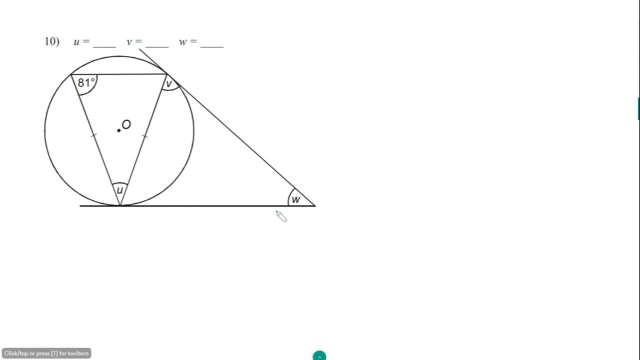 And then we need to find angle v, u and w. Alright, let's see what we can do. First, we know here it's going to be x1.. Why? Because these two legs are equal, so the base angle should be equal, okay. 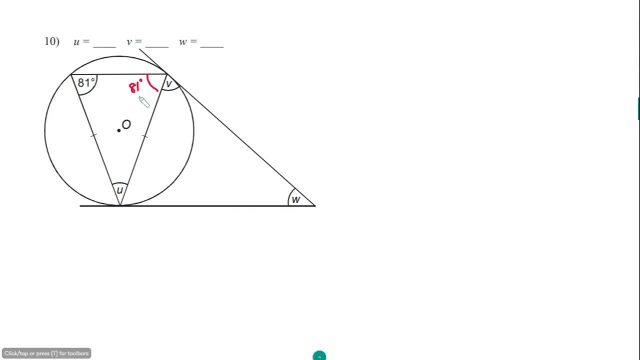 So it's easy for me to find angle u because I have a triangle. these two angles add up to 180.. So to get angle u, add 81 plus 81,. oh, did I say 1?? Sorry, That's going to be 162.. 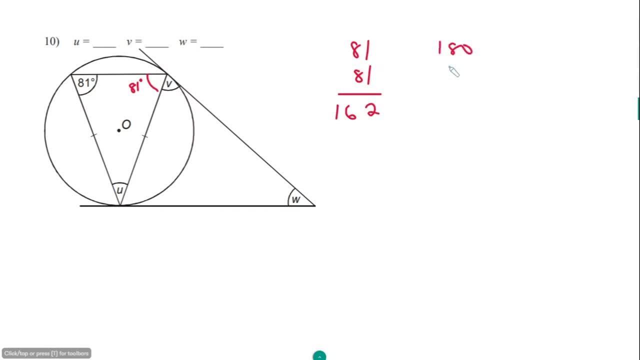 And to get angle u, subtract this value from 180. And that's going to give me 18.. So angle u is going to be 18, 18 degrees here. So angle u is going to be 18 degrees. Next we need to work out the angle v and w. 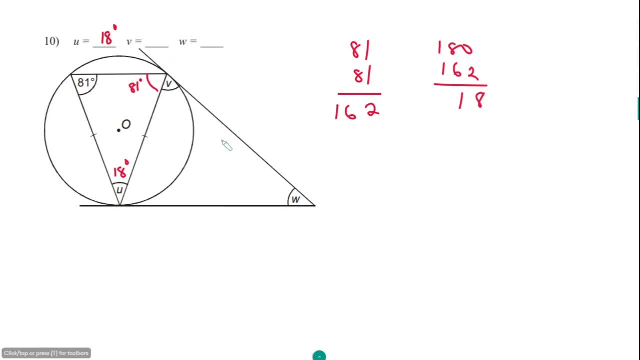 Now already we know that we've got a tangent here and another tangent here. This length here should be equal to this length, meaning that this angle v should also be. this angle here should also be angle v, So they should be equal. base angles are always equal, okay. 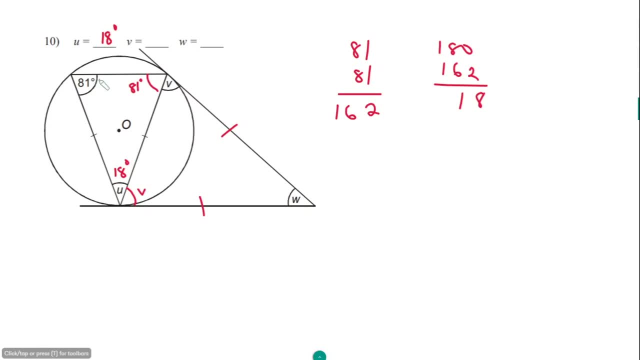 Now we already know that if this angle v is alternate segment to this angle here, so v here is going to be 81. That's quite, very, very slick, okay. So v is 81 degrees here, And if it is 81, this angle here also has to be 81 because, remember, there is a base angle of this triangle, okay. 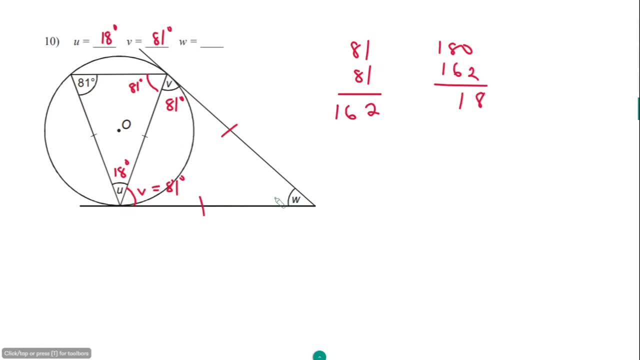 So to get w, add up these three angles to be 180.. So to get w, I need to add these two angles First. that's 81, add 81.. 81, add 81,, that's 162.. 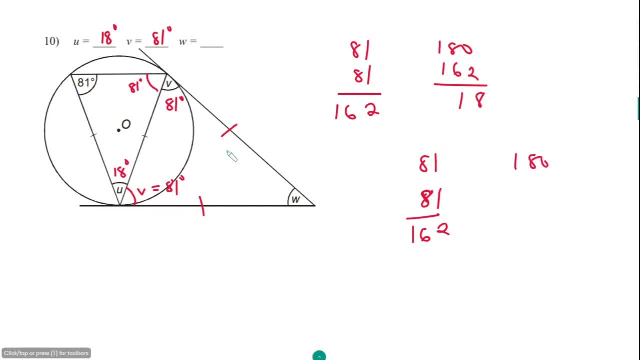 And to get w, I'm going to subtract this value from 180 because, remember, there's some angles in the triangle. that's 180.. So 180, subtract 162, that's going to give me also 18 degrees. So w is 18 degrees. 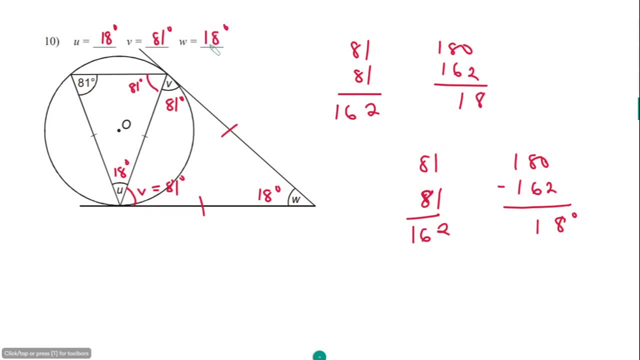 Wow, this is. I hope you enjoyed this video And if you like the video, like and subscribe to this button. Have a great day. 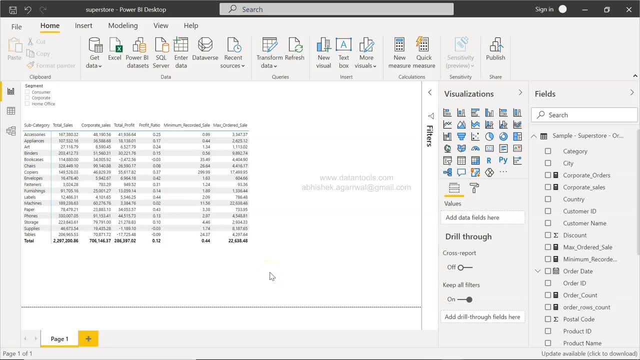 hello there and welcome to the new power bi tutorial video, and in this video i will show you how you can apply the power bi tax function average. so average is something that you will use quite a lot in your reports and dashboard as it gives the measures like average sales average. 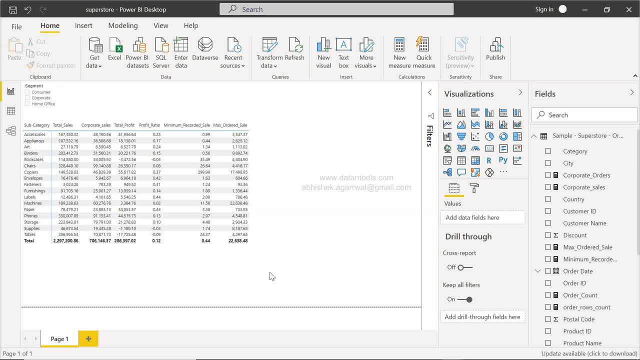 order, quantity, average profit. so whatever value that you are having, it gives you the average. and why it is important is because most of the time, whenever we want to look at, let's say, along with the total sum or the percentages, average is also one of the key measure which basically gives a 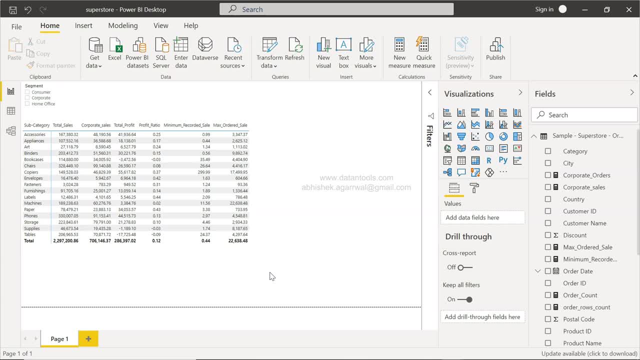 ballpark figure as to how we are doing when we are looking at our business metrics, and that's why many times it is present in our reports and dashboards along with the other metrics. so i will show you how you can create it and, before that, quick information about the the three links which is present in the description. one is the data set.